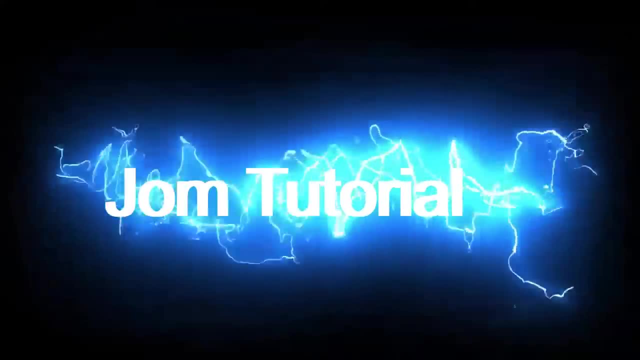 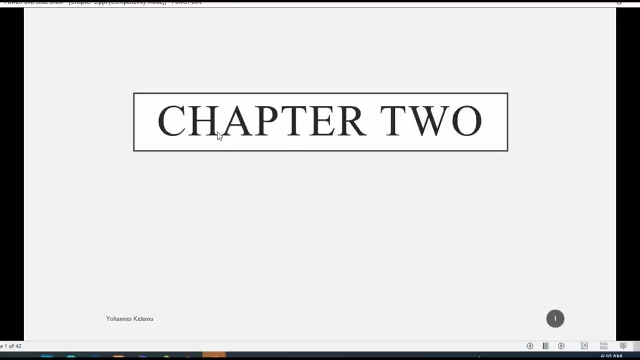 Hello everyone. welcome to the next point, chapter 2, which is the chapter 2 of the Concurrency Control Technique. The Concurrency Control Technique is used in chapter 1 of the Transaction: Concurrency Problems Lost, Update, Demo, Temporary Update, Incorrect Summary and Concurrency Transaction. 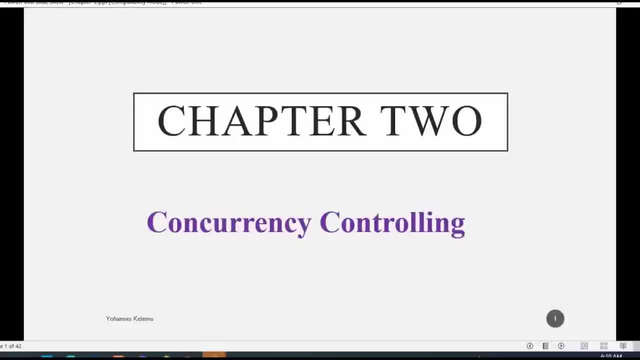 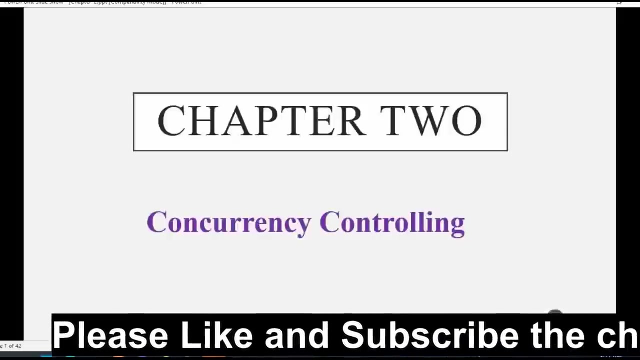 These are the main problems of the Transaction Concurrency Control Technique. So the Concurrency Control Technique is a very important concept. In order to apply the Concurrency Transaction, we need to learn the technique of the Transaction Concurrency. If you are new here, please subscribe to the channel and click the bell icon. 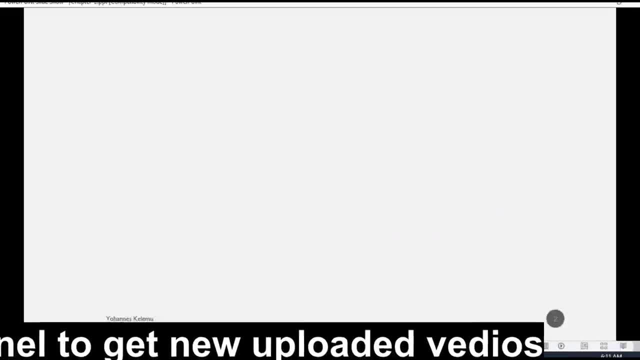 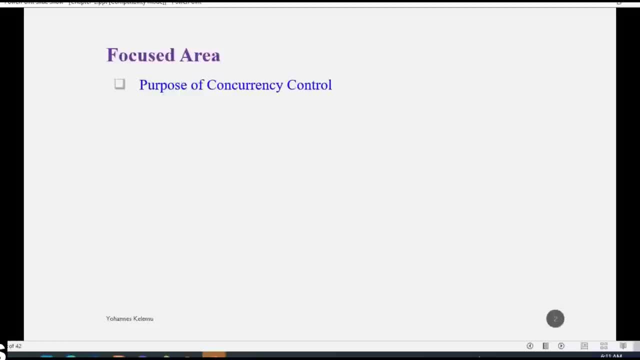 So this chapter will focus on three main topics. The first one, the purpose of the Concurrency Control. The purpose of the Concurrency Control mean to know concurrency control techniques in Manila, to like in the locking, in the timestamp, in the optimistic multiversion and look grand. 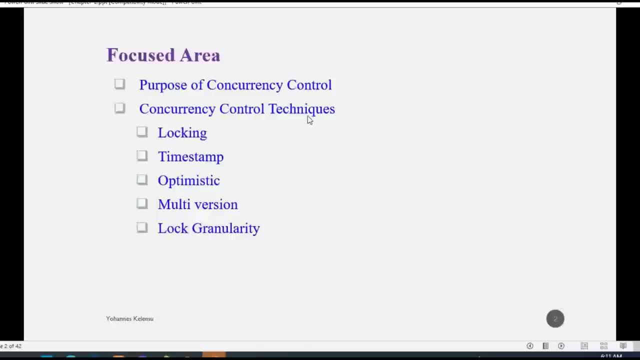 and granularity and mineral. yeah, concurrency control technique in Manila to nacho green as in one by one. yeah, you need a little more than no. so introduction in the transaction processor in Manila. like the transaction processor, divided into two bullet, make a fellow. the first one, concurrency control. 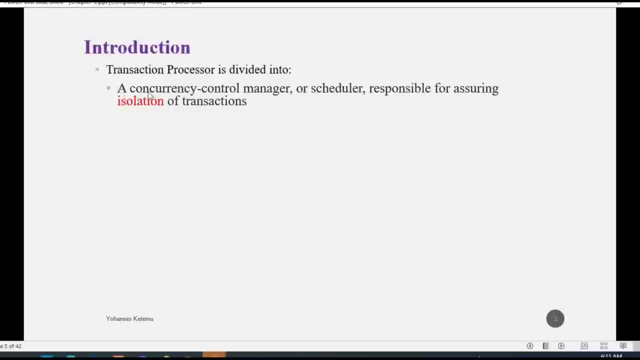 manager will the most K? Judah Manila. concurrency control manager scheduled a mallet responsibilities for assuring isolation for transaction transaction conflict and I know order transaction ordering is a little agree. concurrency control manager Manila. the second processor logging with no more recovery. manager Manila, he logged in with the same procedure, the same procedure, the same process. 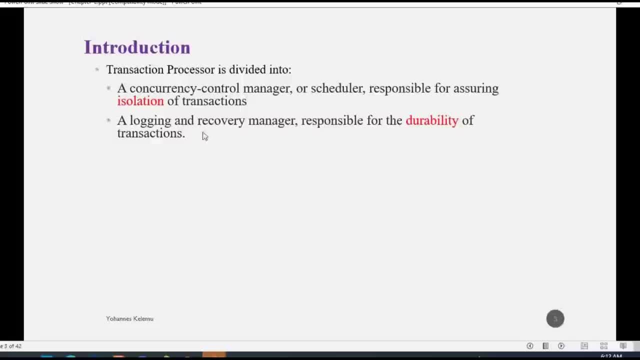 login recovery manager, responsible for the durability of transaction. in transaction gravity we don't recover ability, uh, uh. so angry scheduler manager, manager must assure that uh, trans, uh, the individual action of multiple transactions, are executed in order: multiple transactions. so the net effect of the uh, the net effect of uh, is the same as if the transaction had. 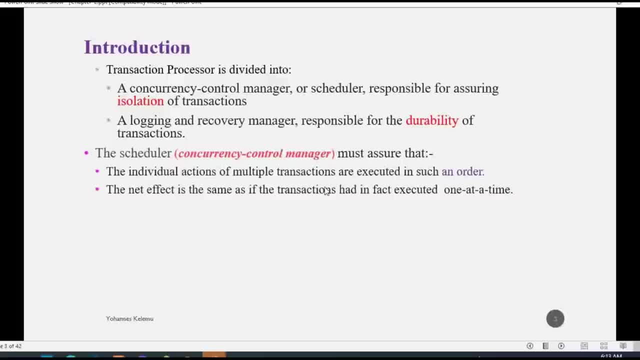 in fact, execute one at a time. yeah, multiple transactions role, uh, concurrency, uh, transaction role, another concurrency transaction and multiple transaction order to set watch. execute your manager. go now one by one. execute your manager. go to my side. need linear checker bar. so let's say net color, yeah, or the nose kid. you know my problem. 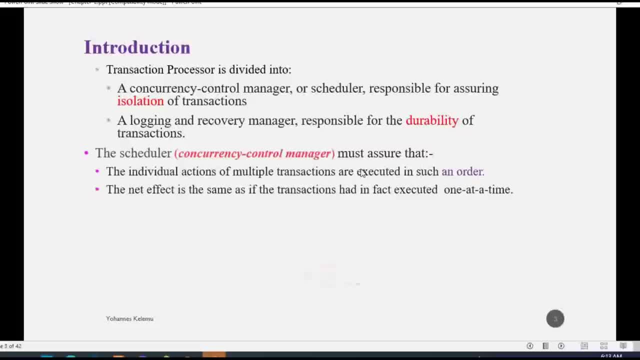 so let's see the nemesis concurrency control manager diagram. uh, meter item. oh, excuse me miracle. oh, next item, excuse me, miracle man, you know e tech transaction model me on in mezzanine or octave limit lot kilo team, don't want me come at all be. 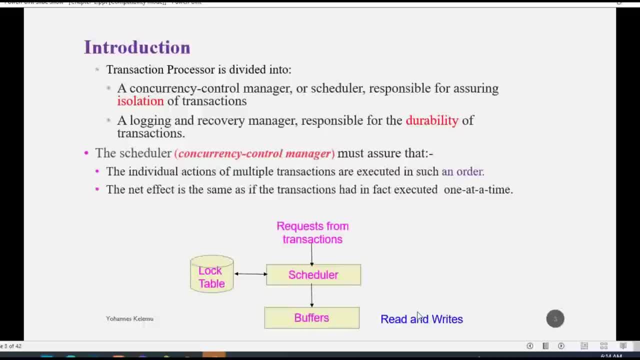 further and get a better life: read, write a menace, commit about. read, write operation. the MNAC I'd bet over and at the transaction introduction: a male, no Lezika. and transactionally boomeru schedule me set out of a scheduler- no scheduler. look TV, read the gamma, look table on locating meter ago paper. 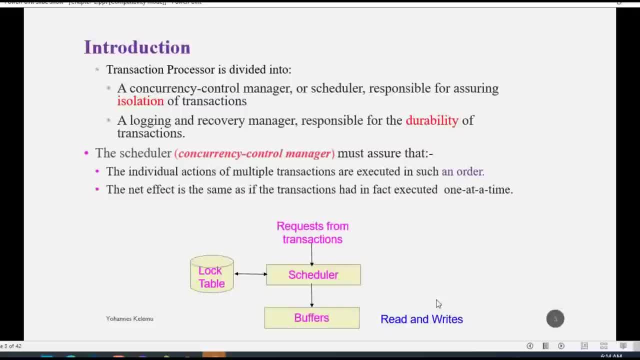 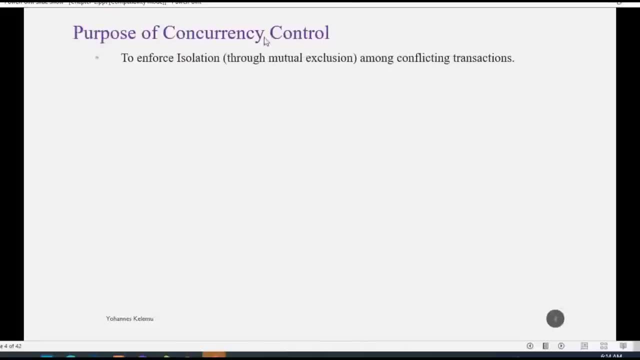 Lino green man in your own read: write operation per four meter ago paper. so what are the purpose of concurrency control? the first one: to enforce isolation. great solution is to enforce the conflict, resolve conflict resolve interference between the transaction. by transaction. it minimizes the interference. to prevent database consistency. 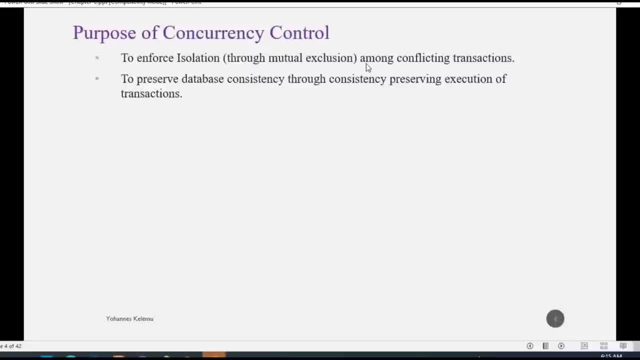 before transaction and after transaction, the database is consistent. the last one to resolve: read, write, read, write, conflict, temporary update, lost, update problem, write problem, and you get the conclusion. what is the purpose of concurrency control, for example, in concurrency execution environment? if someone conflicts with you, you have a conflict. 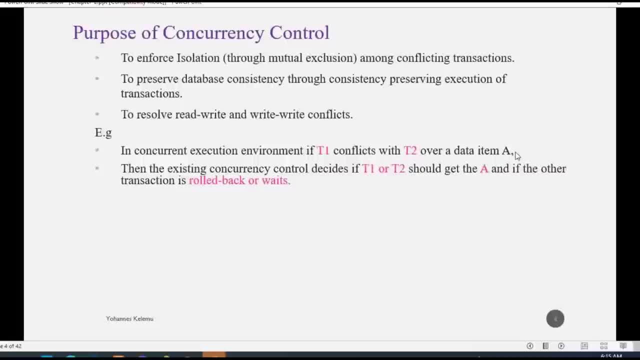 with Bifetro to access the database- the item N. then the concurrency control decides what to do. if you or you should get the item A, the item N, what will happen to you? So if you have the same criteria, the probability of getting a rollback is the same. 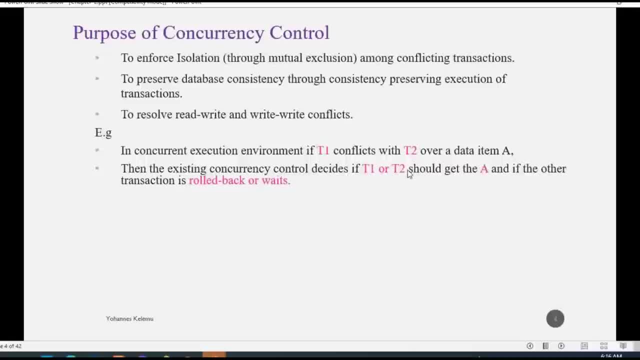 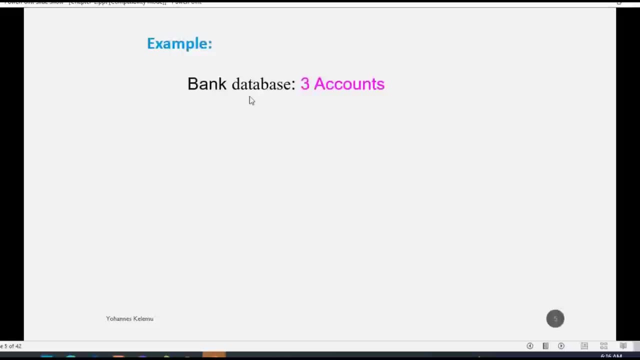 For example, if you have access to an item, the probability of getting a rollback is the same. This is called Concurrency Control. For example, let's say you have a bank database. The bank database has a source account. The account is A, B and C. 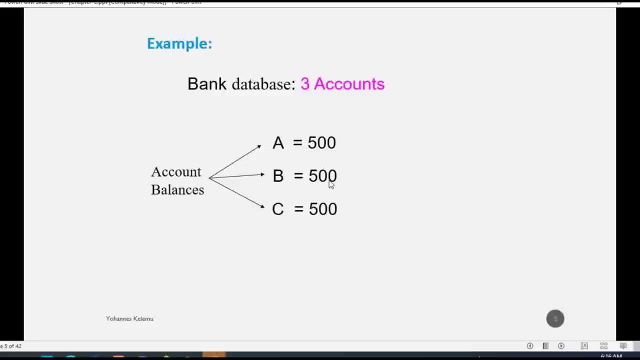 Account A is 50% B, Account B is 50% B, Account C is 50% B. So the property, for example, is A plus B plus C. The source account is 100% B, For example. this is the same. 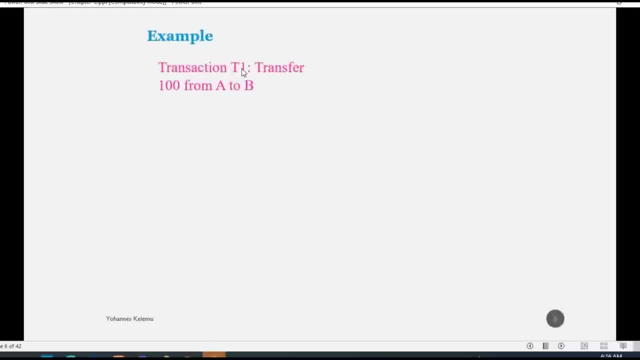 In this case the transaction is transfer 100 from A to B. So would A be the transfer number to transaction 1? So this number starts from A. Then, by entering the value in the middle, the number starts to go up and the value increases. 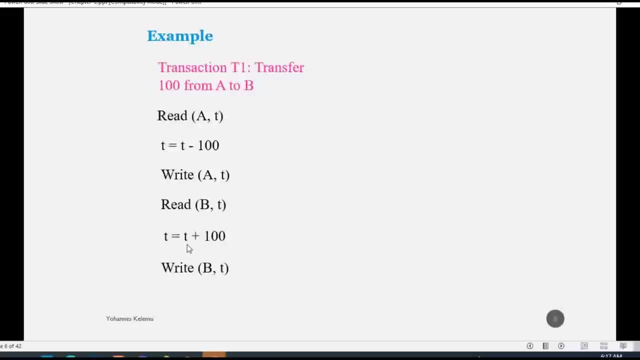 This is called an update. So when the value changes to account B, this is called balancing. So by entering the number the number increases. So this place for A is transferred here. So this is called an update. transfer 100 from A to C. 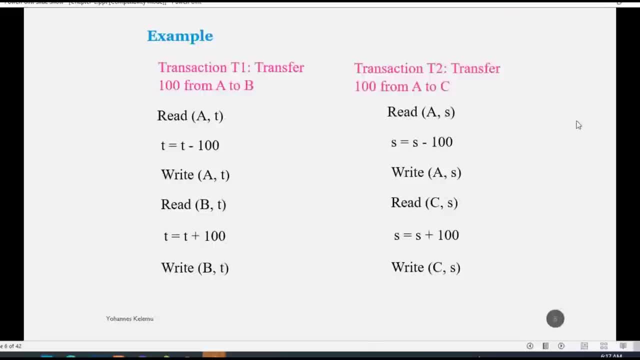 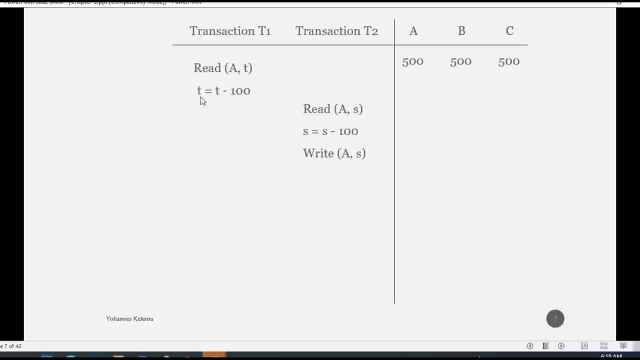 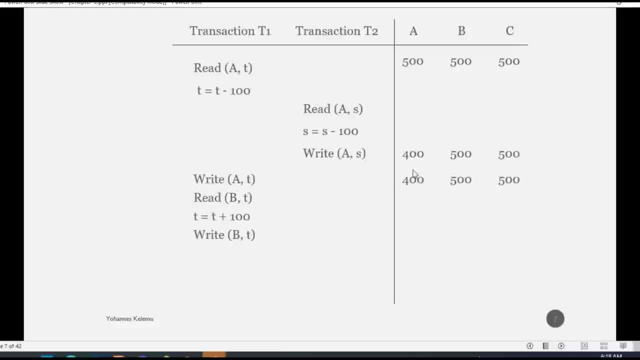 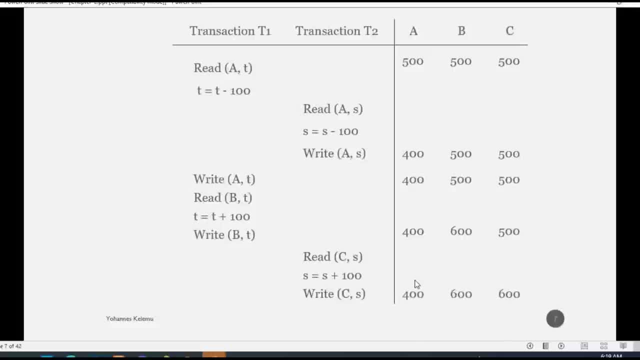 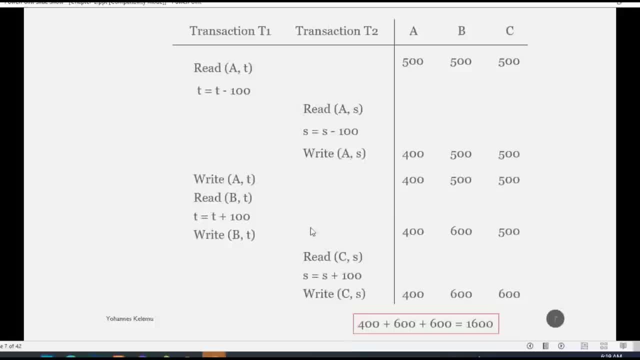 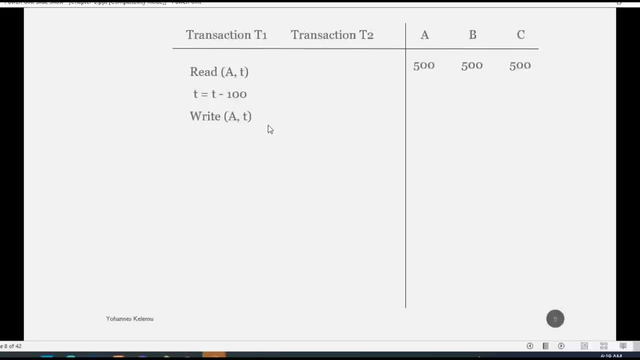 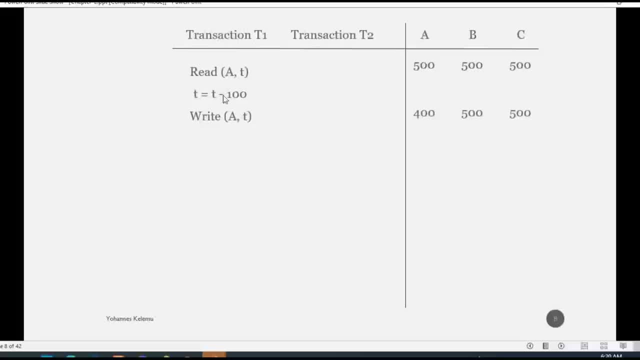 We need to know the date of the transaction. We need to calculate the minute system In order so we can know the minute time. So let's say there is a minute, It's our money. We need to find the minute system And if we find it, we can more or less knowing that it is the minute process. 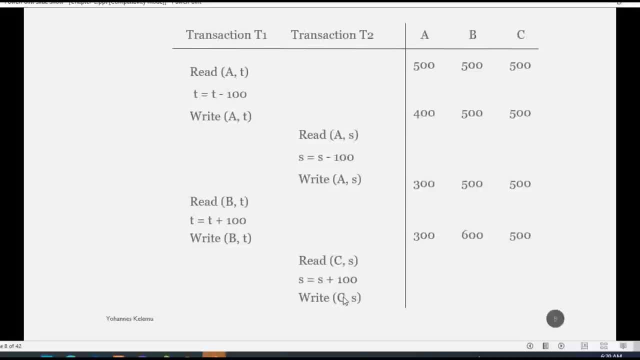 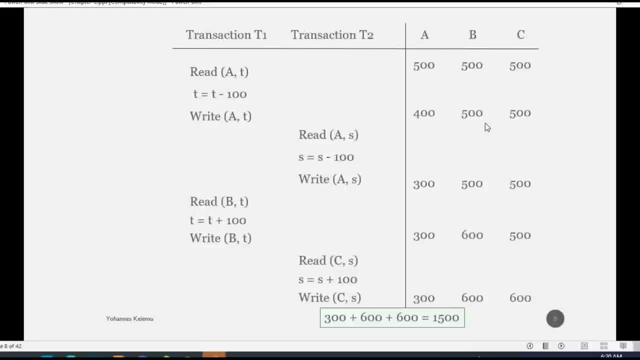 Before transaction and after transaction The sum equals the database consistency, So this is called interleaving serializability, Interleaving serializability transaction. As you can see, the database consistency is like a conflict, So this is called the schedule. 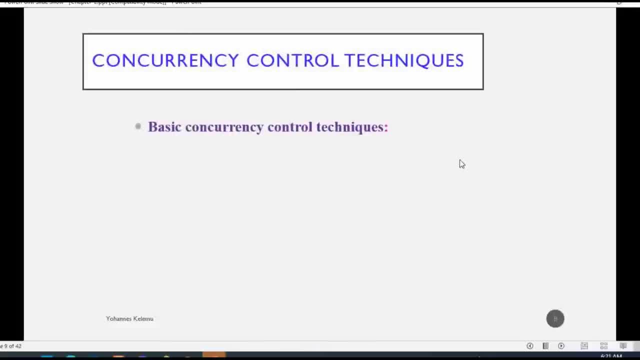 This is called the concurrency control technique. So what is this concurrency control technique? It is a locking, timestamp and optimistic method. Locking is like this. So what we are going to do is we are going to use the conservative approach. 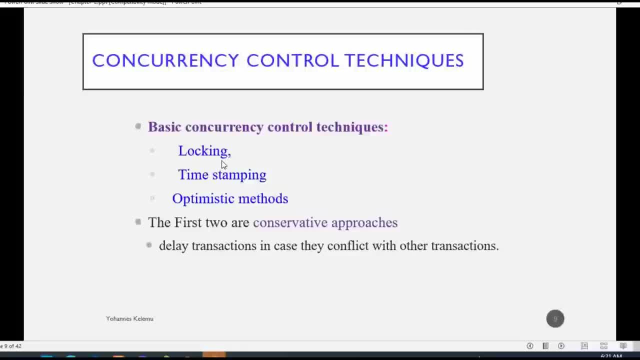 We are going to use a delay transaction in this case, So we are going to use a delay after the execution. This is the optimistic method, but there is a conservative future, So we are going to use a lock and execute method. 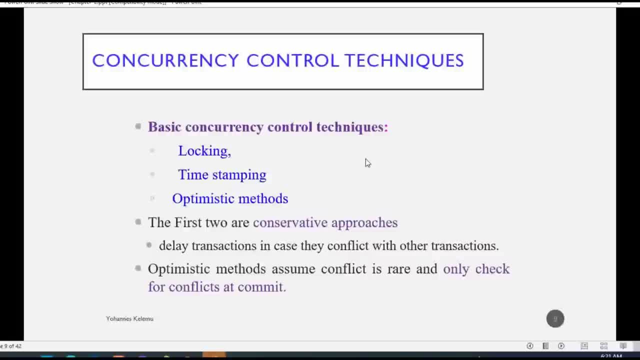 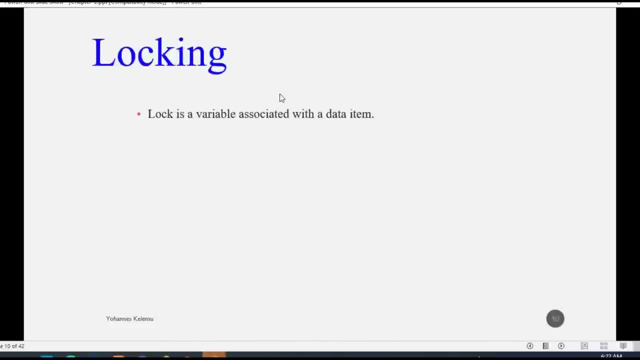 We will use the transaction execute method. So we are going to use a lock and execute method. This is a free code of execution. minimum minute conservative. feature in the minute delay problem: me panagher, yellow, modern, so angry Zika. locking technique: nailing the locking. 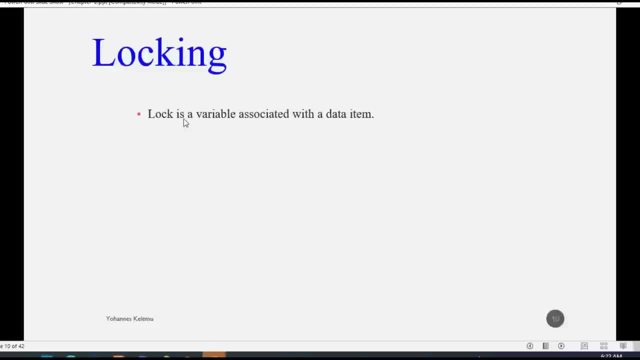 concurrency control minima. that no. locking- my letting me look- is a variable associated with that item under that item. lock: moderate- mess got my asthma. no. describe the status of the data item with respect to the possibility operation that can be applied to each degree: possibility, operational and item. 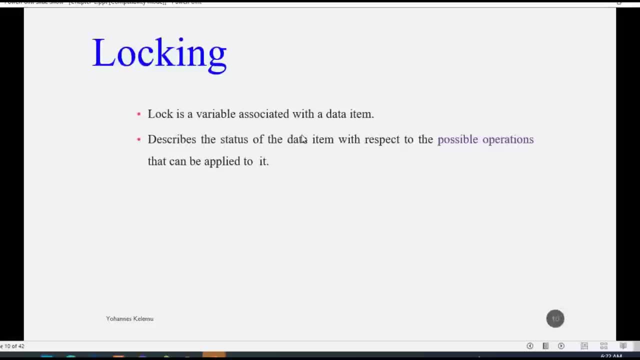 right, look, which I would a more read. look neutral, yeah, I'm no possibility, operational, lazy way. right, look, we read. look no blue, or a look at the guns like a reader book, a jealous water. we don't write our culture as a wallah, you like. come on, yeah, I'm gonna. locking you para, loking you para. 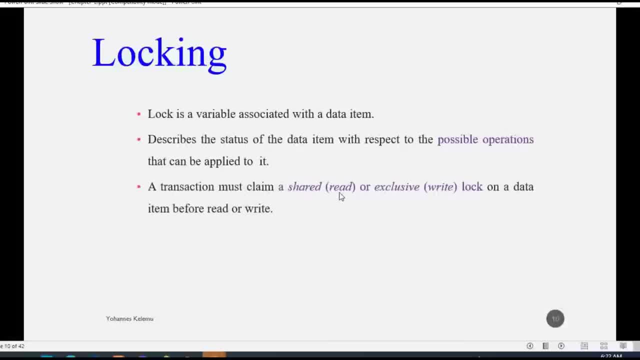 so that is looking bullets. no minkah flow shirt. look when the more it look exclusive, look right, look in a lot of shirt. look when the more exclusive look, read look. look there, members, look narrow crazy operation. security. permission to read or permission to write transaction one read lock. permission to read. 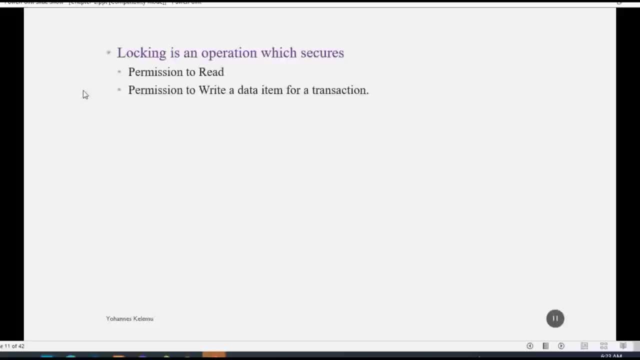 transaction one write lock. permission to write transaction item. update permission to write uh behalf of the requesting transaction, not permission item released in the transaction, and the item is made available to all other transactions and the transaction is executed. and the transaction is executed, we will use the LOCK technique. 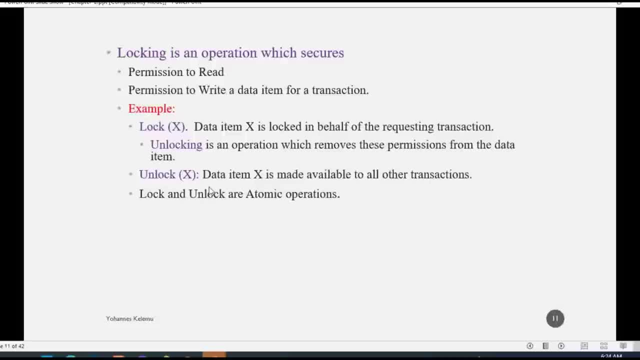 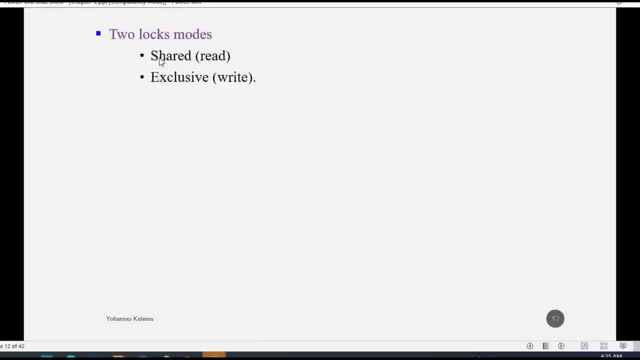 look now, look at the atomic operation of me pilot and they look at it again. sir also took a chair as well. I know I look America, malino's legendary atomic future. yeah, you're not sure. not to malino that look more than the latino Richard. look nice lucy, look man latino. no, Sherlock might read malino exclusive. 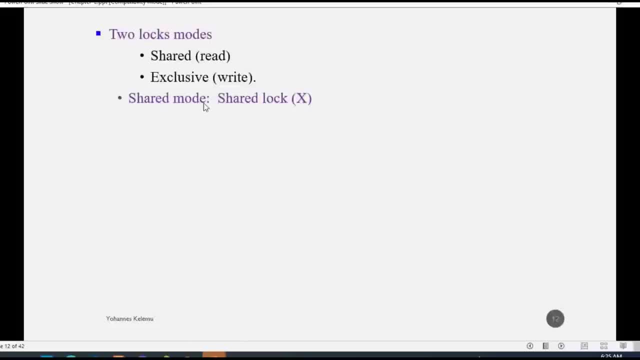 look malit, right malino social shared mode, my just shared. look malino. that means more than one transaction can apply Sherlock on X for reading its bali malino email shirt. look like boozoo transactional chaluk matricula lomano gato read. read layman, a little conflict in the modern shirt might read. 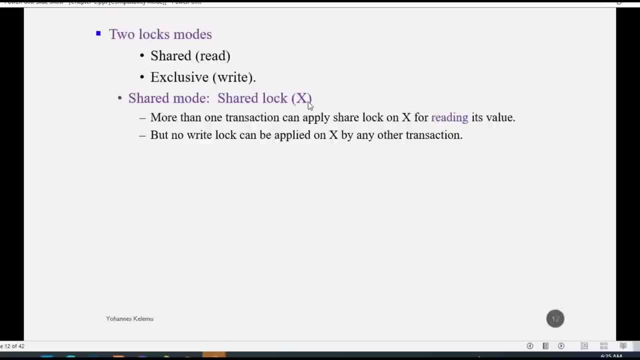 malice Rona. multiple transaction. X in lock. mark each element. Larry's look marvellous. look malino gnarly zika shirt. look like minute right. look mark a challenge the moment my head update swim right operation. my cadential who loom? transaction. I'm sorry, I said transaction which can do 202 t3 alice. 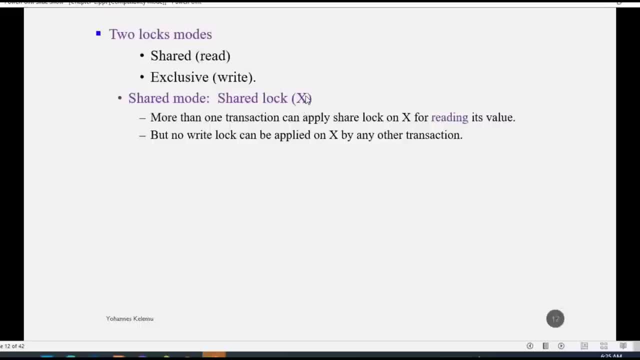 caster as a transaction, Carla X in a serum transaction. look malicia, again a certain transaction room. you know three normal- it's John Reed Martin- which are ready share it. look much on America, right, look in my rega chluma lena exclusive mode calling in right, look malice, right, look malice only. 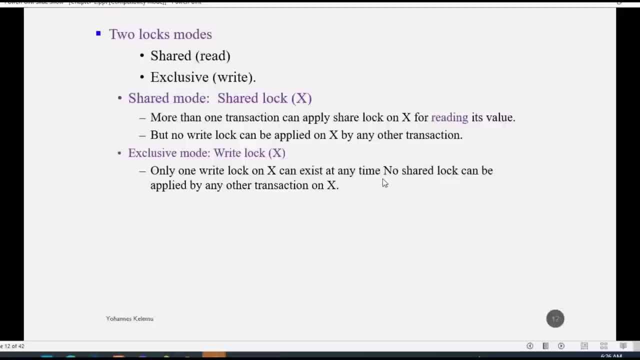 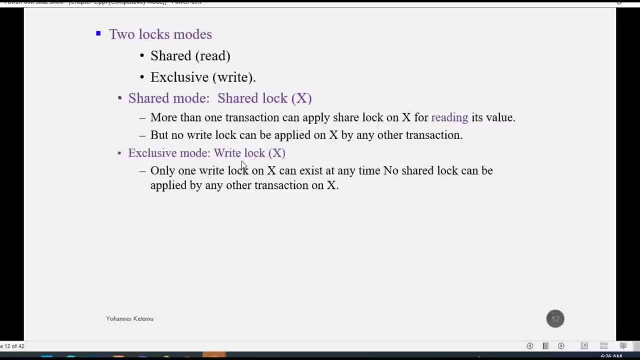 right like conflict. I love learning. look at transaction on tonight and I right right cut it right over conflicting sly see design iron and I tell Itcha지가: look miracle Zigan. to multiple it read: look mar tio auntie garden. and it's a transaction, Pitcha mirMap. 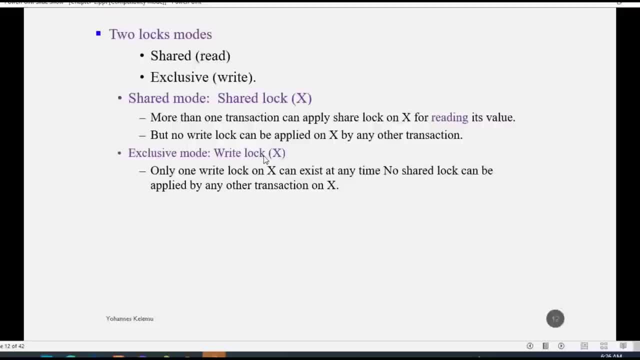 local Martin Charo and transaction Charo, caton. a lot of natural logic about a. So this is exclusive lock. So matrix is a conflict. Read read corner is yes, That means we have a conflict. Read read corner is a conflict. Write read corner is a conflict. 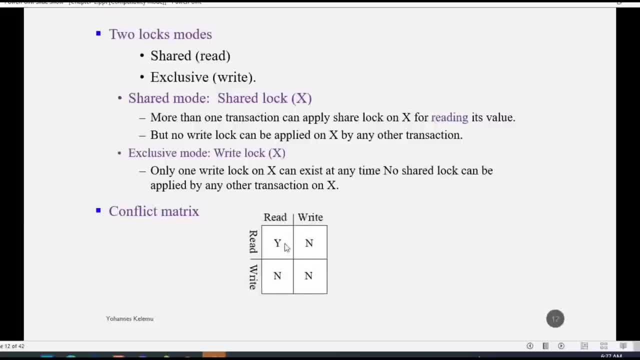 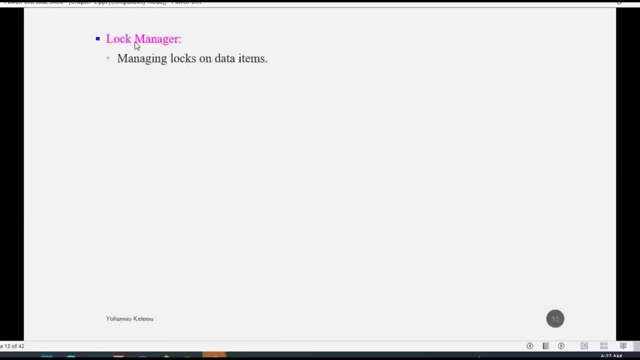 Write- write corner is a conflict. Only conflict is read read corner. So read read corner is not a conflict. Read lock is a multiple transaction. So what is a lock manager? A lock manager is a lock of a data item, Like a scheduler or a buffer. 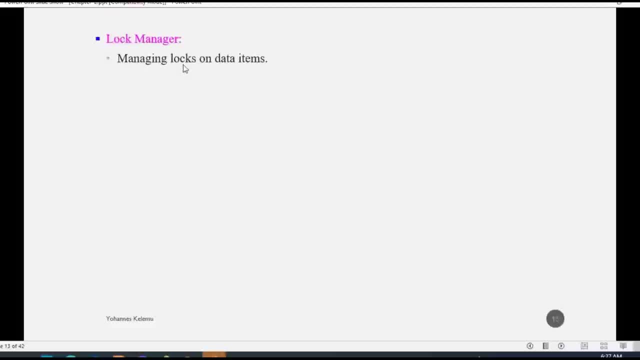 Or a lock table Like a lock that is used to make a transaction. So a lock manager is a lock manager. A lock table is a lock table. A goal is to make a transaction On the lock Enter A lock table means Transaction id is here. Doctor is here. 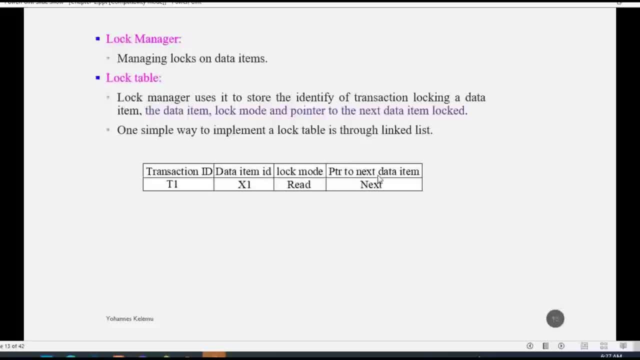 A lock mode is here. pointer to next is here. For example, transaction id is Transaction 1, transaction 1, transaction 3. Here data item id is: Transaction 1 is entered as Lock. Transaction 2 is entered as Lock. Next transaction 3 is entered as lock. 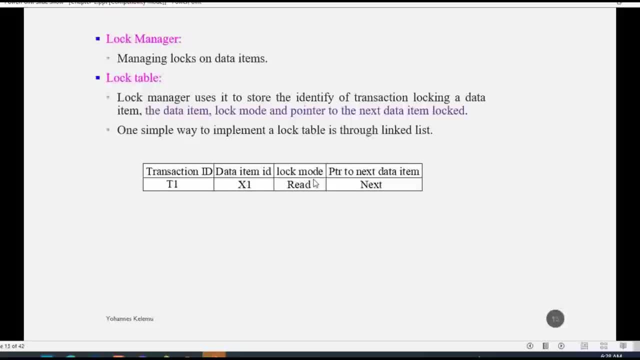 That is called lock mode. lock mode is read lock or write lock. exclusive is short lock. next item is lock lock. transaction 1. next item is lock lock. pointer to next is lock lock. lock table is equal to lock manager. lock manager data base is required that all transactions should be well formed. 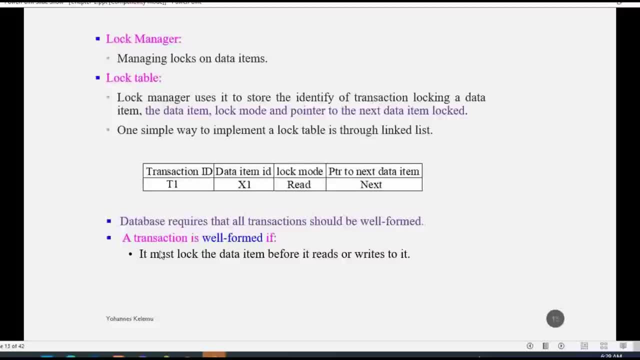 execute command. to execute 메뉴. Ordinal 메뉴 should appear to be awake 메뉴 Shiva should appear to be awake. it must not lock and already locked that item, but it must not try to unlock the free data item. 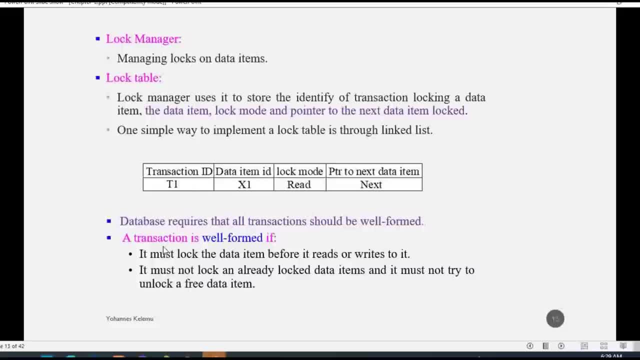 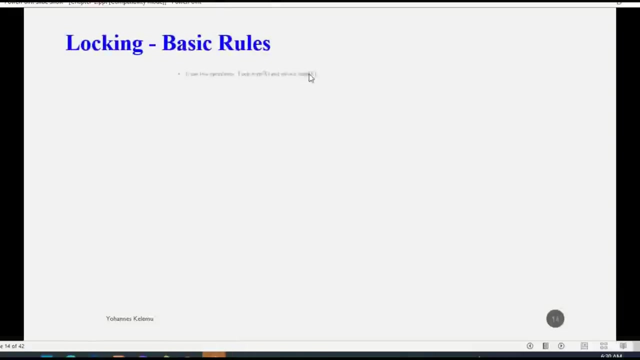 unlock the item must not try to unlock the free item. so we need to know that the transaction is well formed. and we need to know that the transaction is well formed. so we need to know that the transaction is well formed. I will teach you 2 basic locking rules. 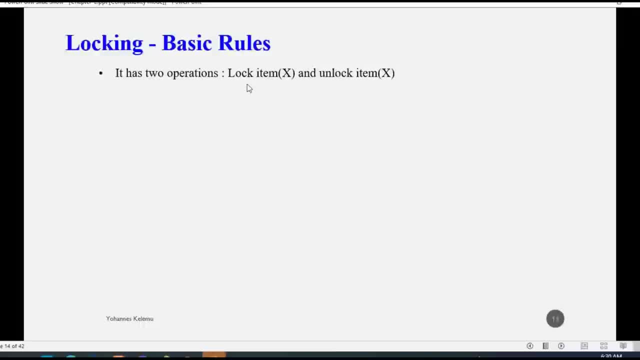 the first means lock item X and lock item X. the other means no locking chances. One transaction may not be locked and lock item X may not lock. log x equals to 1 means x already locked net. log x equals to 0 means x already unlocked net. 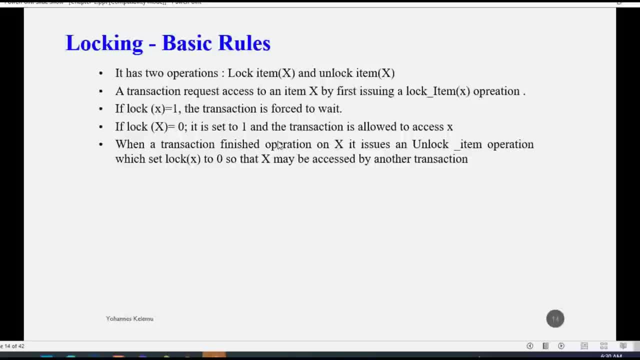 when a transaction finish its operation. when a transaction finish its operation, it will unlock log. x equals to 0 means 0 unlocked net. if transaction has short log, it can read edges and updates. short log is read. short log is updates if transaction put exclusive log. 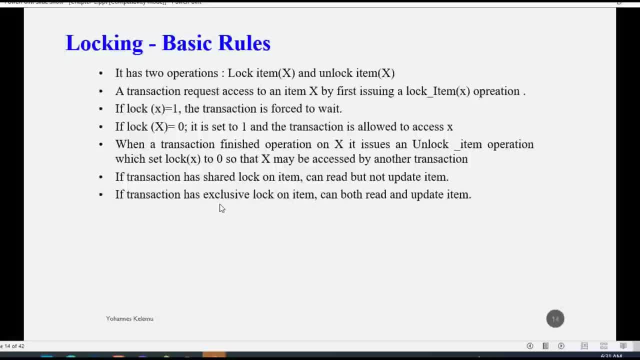 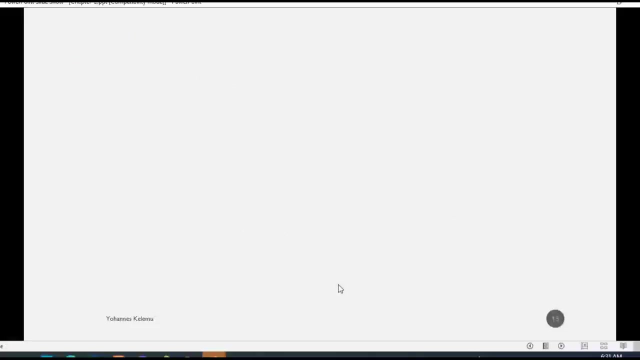 read. it is exclusive, exclusive go 1 at a time. it is read read cannot conflict read lock, read read more than one transaction: lock lock. exclusive lock transaction exclusively access. read lock, read lock. if lock x is equal to unlock one, x is equal to read lock. 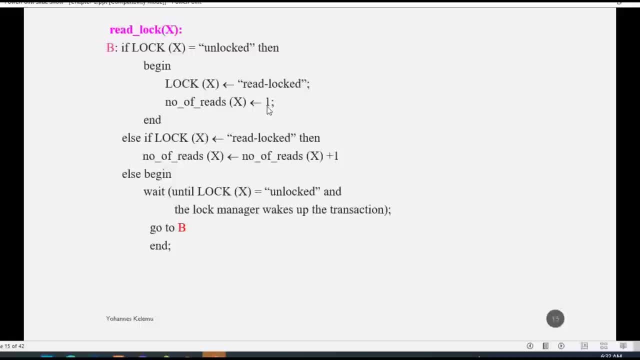 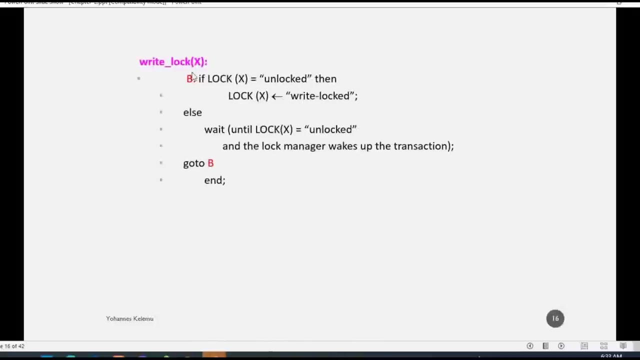 read lock. read lock is the number of read lock plus one, that means transaction one. then else, if read lock is the number of read lock plus one, that means action item, multiple transaction, read lock plus one, then right lock exclusive lock, right lock x lock if lock x. 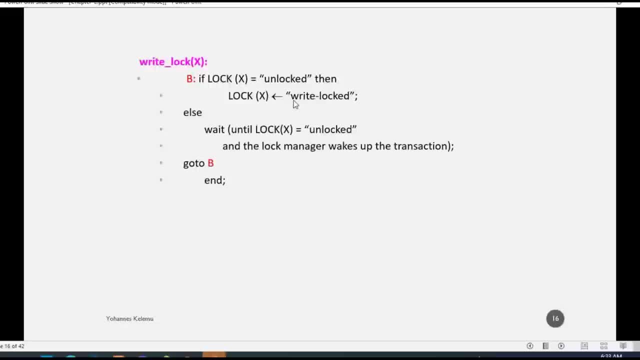 right lock unless x lock done. test power, ufc lock conversion log upgrade. the most important because the unlock lock. We need to change our read lock to the right lock. We need to create an item that we can use in the transaction, For example, if the transaction number is X. 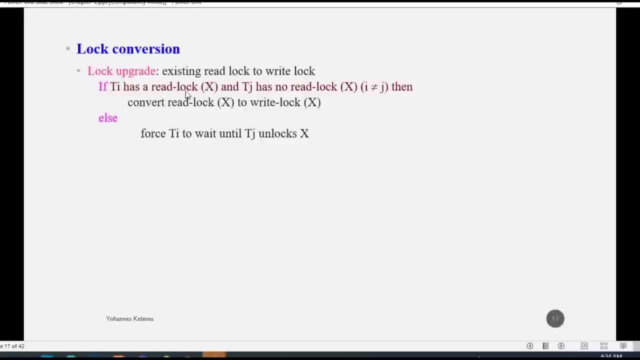 and the transaction number is 2, we need to change the read lock to the right lock So we can see that the transaction is not the same as the previous one. So we can see that the red lock is the same as the red lock. 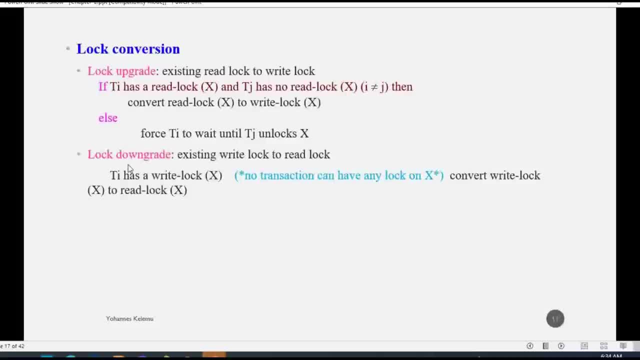 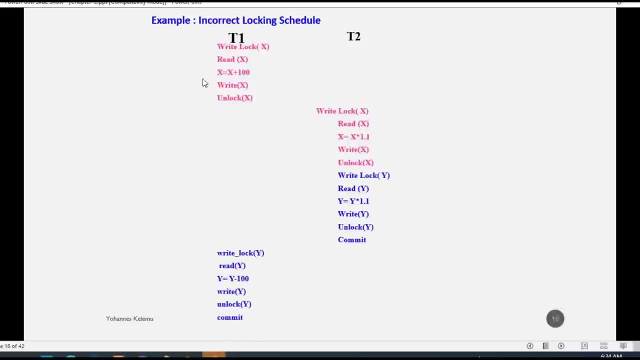 So this is called lock upgrade. Lock downgrade is the same as the red lock, So this is called lock downgrade. So, for example, we have the incorrect locking schedule. This is the incorrect lock scheduling. Because this is incorrect scheduling. 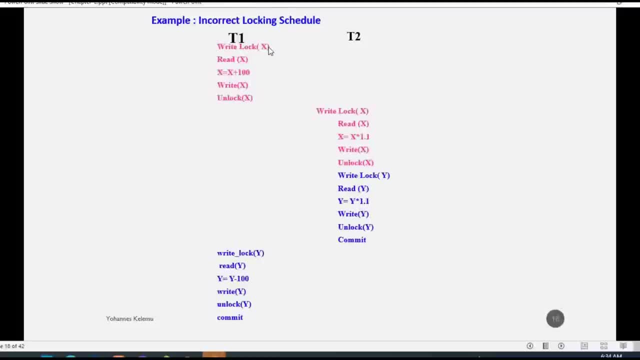 Here we will change the red lock to x, Then right x to x plus 100, then right x to x plus 100. We will change this to unlocked lock. Let's go ahead. So we are going to write x in the right look. 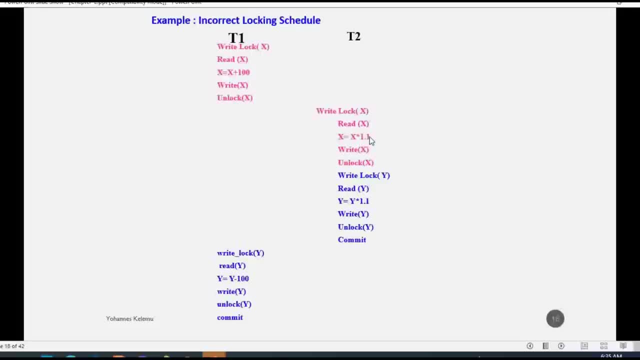 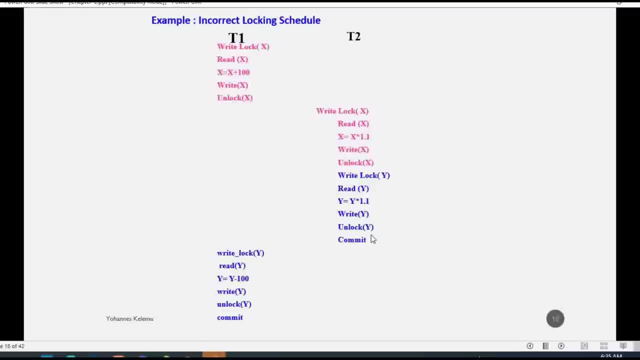 Then write x in the right look. Then write x in the right look And I'll tell you why I call it as incorrect look. Now you know what is incorrect look And I'll tell you what is two-phase look Look can look like this: 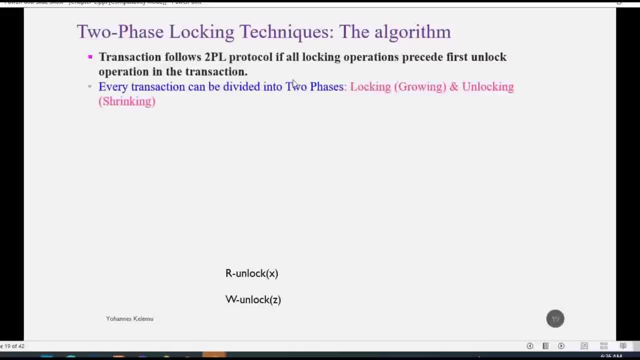 the token wallet he took his look. technique man, technical Charlo, looking when the mug ground, growing, now unlucky when sharing come in a lot, looking when growing and looking when sharing come in a low. and the model not looking when growing management, no, a transaction apply. look read, look in right, look on. 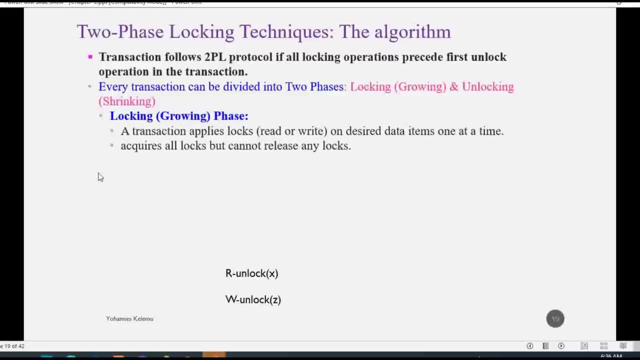 a desire data item, one at a time, acquire all looks but cannot release any lock modern ones. you come in the know any transaction, execute murder. come a general benefit. me fellow got shown that was my mother got a bit. look, mother got a bit. what a unlock comic about perfect man who look at it a wallah with a 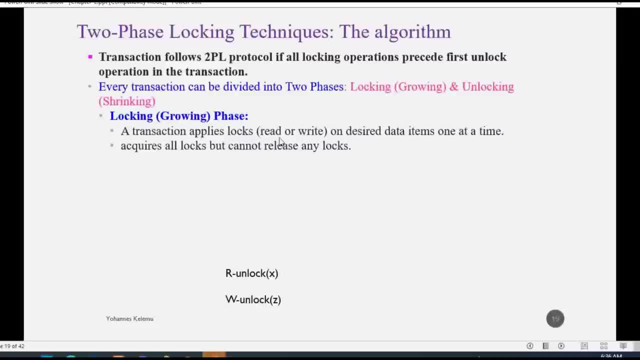 mini-gawa would unlock a glass lady. look, pull them. that was looking at it. but way looking grew and I'm a growing face nominal unlocking where the more sharing phasing laws. you got a look at it. I got shown. item was unlock my reticent. 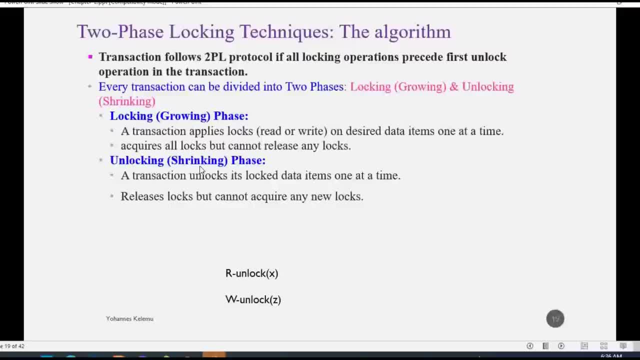 unlock my reticent, unlock, my reticent jammer. you mean no, mano, unlock inłem sharing face nominal. look is he got the guy I said night. let me say like this: I got transaction to all my bad, the transaction Allah, these transaction exit wine. they didn't. 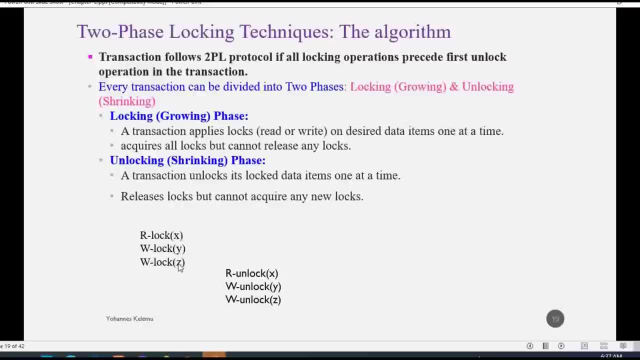 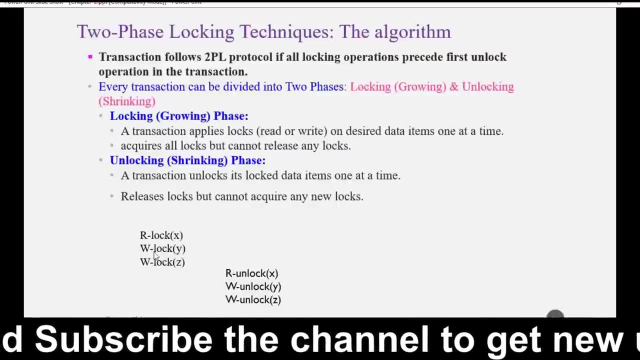 execute my reggie feliga, let me action wine. that didn't excuse my recline, fell like direct me matoo accident wine, a little bloke and regard mahler blocker again, For example. if you want to execute the command, you have to do the following steps. 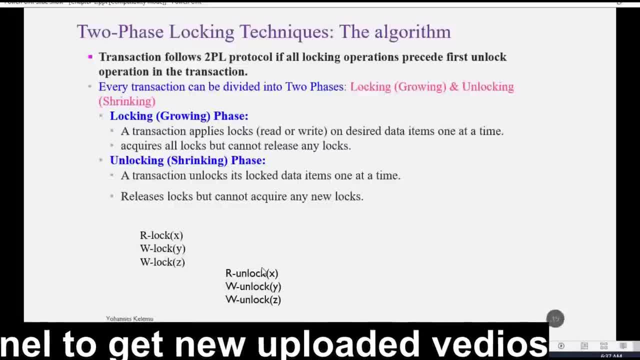 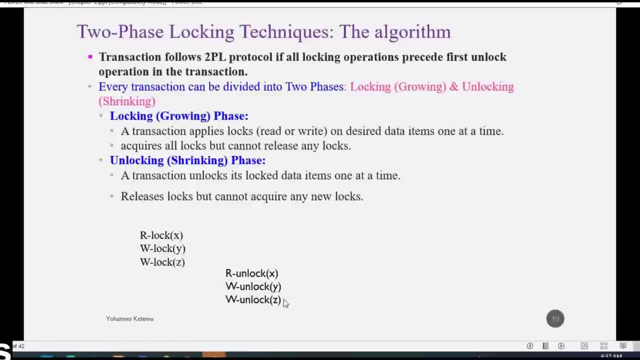 First you have to do unlock. When you execute the command, you have to do unlock. When you execute y, you have to do unlock. When you execute z, you have to do unlock. So this is called the growing phase. 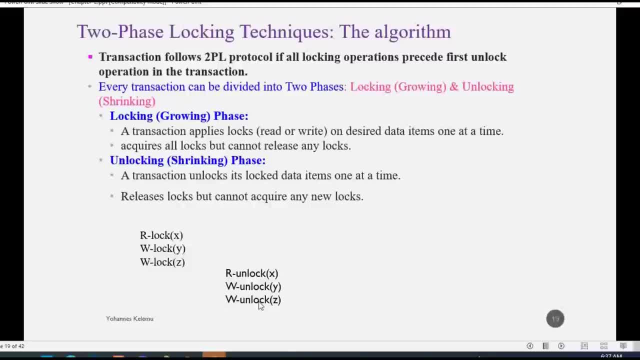 Second, you have to do the unlock, which is the shrink phase. This is called the design problem happening data: When you do a transaction, the data you're getting is unlocked and then unlocked. So this is called the growing phase and the shrink phase. 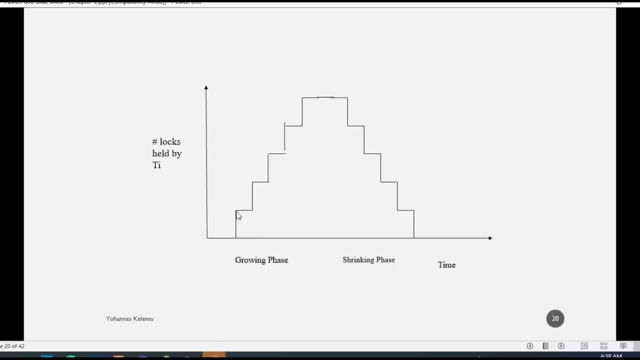 For example, I try to do the growing phase and it's not unlocked. Let's look at some data. So if you want to execute a lock, you need to do a shrink phase run. This is a diagram of a two-phase lock. 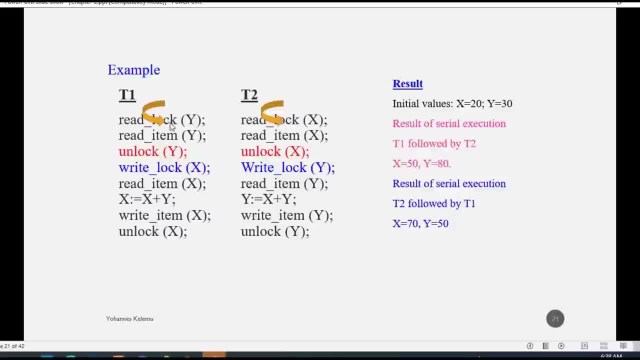 So, for example, read lock is 1, read item is 1, and unlock is 1, read lock is 1, right lock is 1, and unlock is 1.. So what is the result? Unlock is 1, read lock is 1, unlock is 1, right lock is 1, and unlock is 1.. 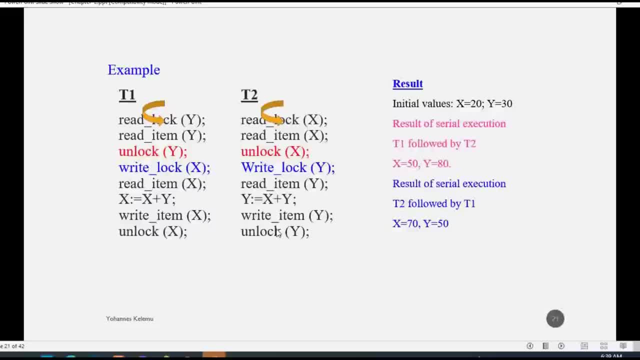 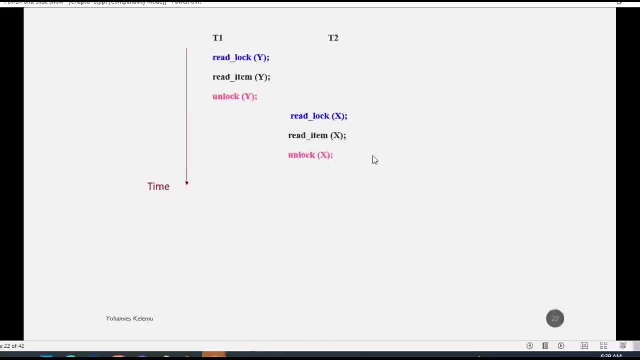 This is a two-phase lock. Another example is parallel execution: Parallel execution. So the two-phase lock is a parallel execution. So the two-phase lock is a parallel execution. So the two-phase lock is a parallel execution. Now let's see if a serializable transaction, a concurrency transaction, is a two-phase lock. 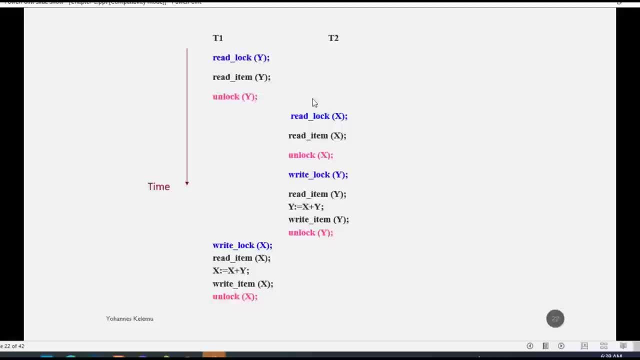 read: look a little, look at it again. Tito demo read: look a little, look at it again. right, look a little, look at it again. Now I'm going to talk about the schedule. Tito, I'm going to tell you about the schedule. Tito is going to teach you how to read. a little, look at it again. 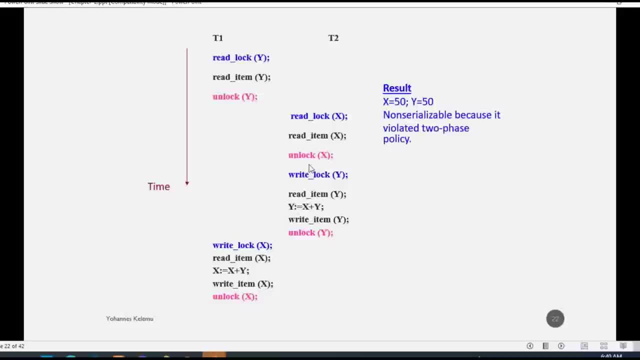 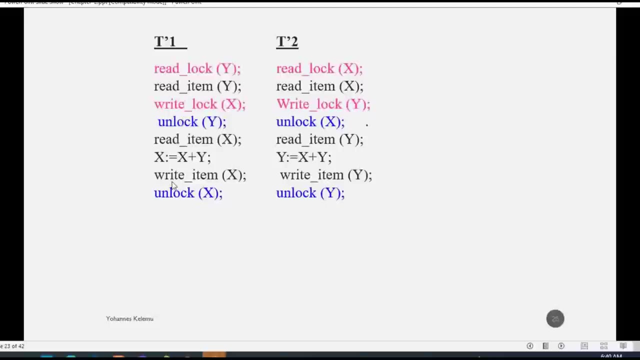 So what is the schedule? If you are applying for two-phase lock, you will not be able to get a serialized lock. In this case, you will have to choose between read lock, write lock, unlock and unlock. This is called two-phase lock or serialized lock. 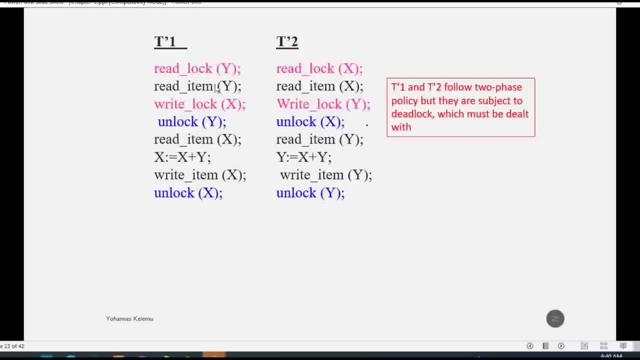 The police will decide whether to satisfy the two-phase lock or not. The two-phase lock is read lock. In the case of read lock, there are two types of locks. One is the read lock, one is the unlock lock. So the three types of locks are read lock. 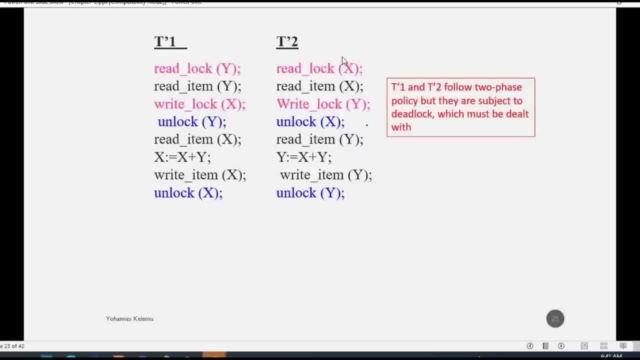 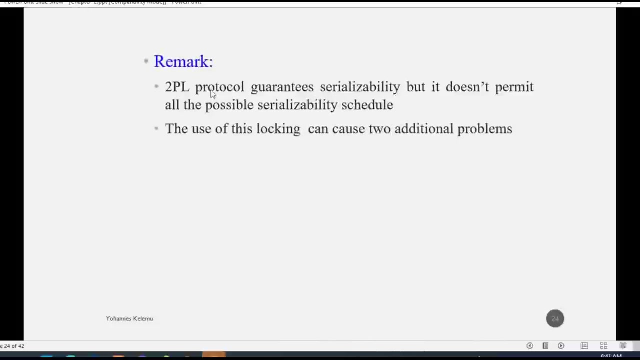 exe, t2 exe, unlock t2, y x. unlock x, x, x x x x. problem in life at that to face look protocol guy and guarantee serialize ability. but it does not permit all the possibilities currently. design did look and I know man and that schedule met a kamala been to face look with serial. 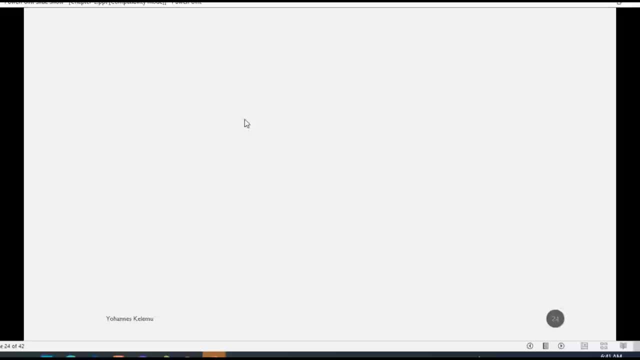 as evil Mona Lepiton- I'm sorry, I'm Mariah, you know, Zika. to face look now negative, not necessarily as evil, added Lamar, Mary, Mark, climate nominal to face look or not terrible as evil Mona Labrador, as evil Mona lab tlz to you. this look can cause to additional problems, daily, day, phase to phase, local. 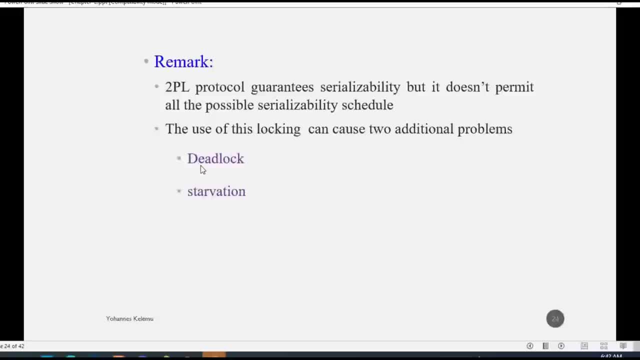 reactions. a flame did local starvation like, got image that did look, not transformation. it to face look mean problem. similarی main problem in Latin such a did look my, let's agree. did look my tomorrow. it's a state that may result when two or more transaction are each way for love. 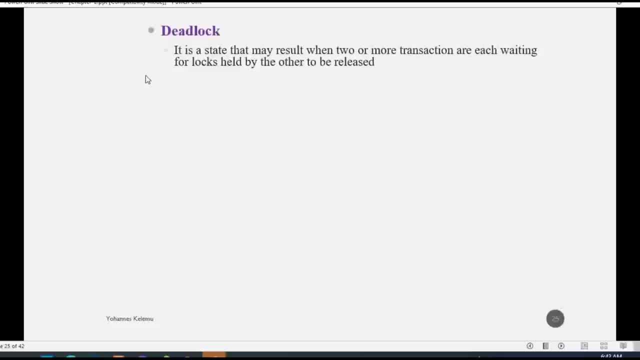 So if you have a deadlock, you can use deadlock as a transaction. If you have a transaction, you can use it as a skill. If you have a transaction, you can use it as a skill. The problem with deadlock is, For example: 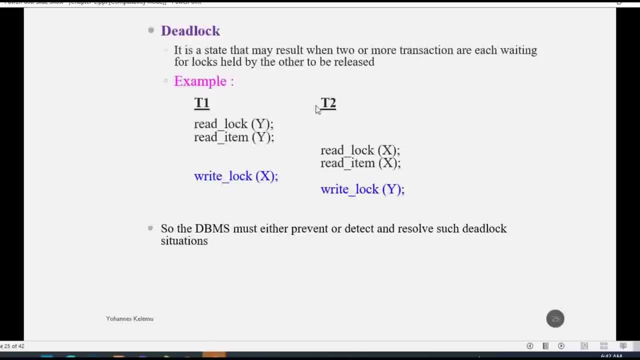 You can use it as a method While you are using a deadlock. You can use it as a trade. You can use it as a trade While you are using a deadlock, So, which means You have to use the deadlock as a trade, For example, when you are using 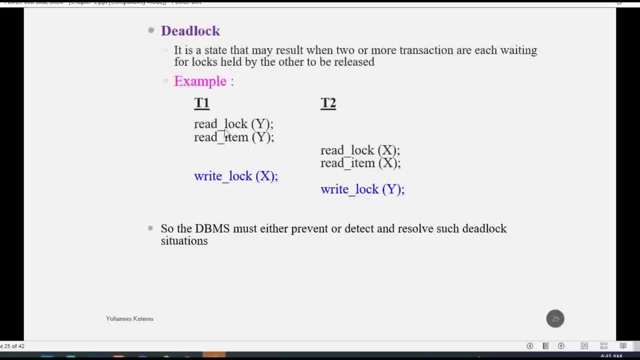 You have to use the deadlock as a trade. So when you are using, the problem is data is not deadlocked and the problem is not deadlocked. and in this case, Data Waste Management System must either prevent or detect and resolve these types of deadlocks. 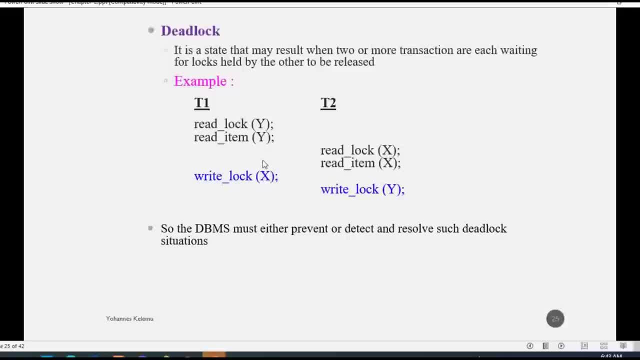 when Data Waste Management System is responsible for the problem. if there is a problem, then Data Waste Management System will solve the problem. failure: galway the move and to a port in the rollback in the other. get one, I know, okay, agree. solution: the Senate Megan right. 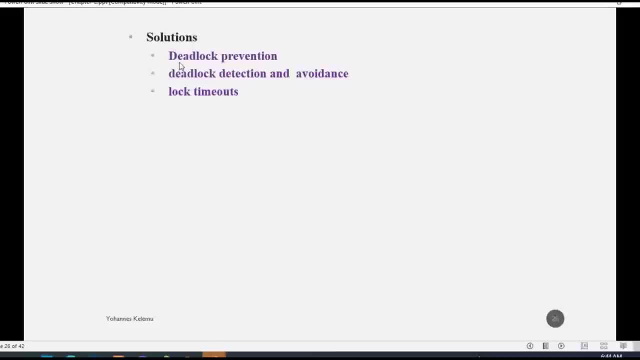 the pack a solution. I don't need it looking pretty much America and then you're it. look prevention, let me look detection and avoidance and look time out to me. follow our loop and we did. look pretty should lie to possibility solid. the first one, the conservative to face, look modern conservative. the 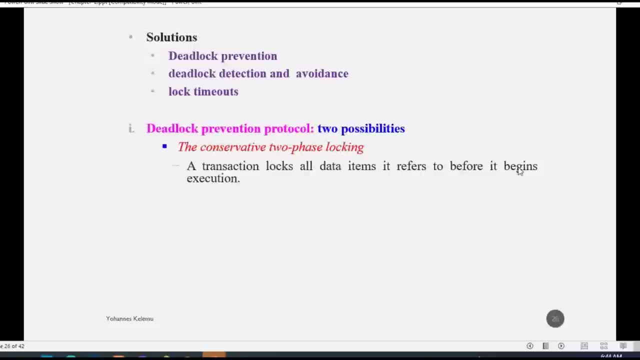 transaction. look all that item it refers to before it begins to execution: Marlena and item execute camaraderie. but it couldn't am if I look at your item watch and look my regalia. but excuse my rick and my general activity, but I'm conservative, you know they look to die. take a mousse. 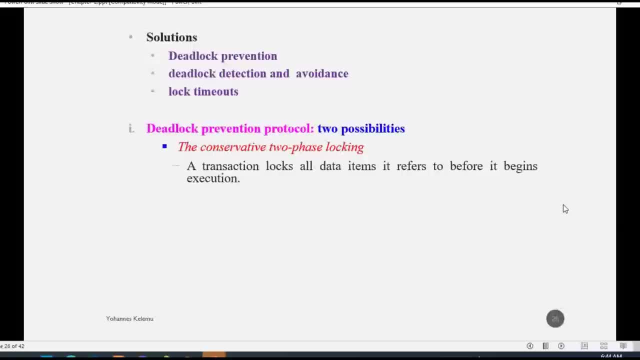 or to catch a lot of angry in the Senate emoji. a look at your media and the conservative to face look in the wallet. so, as a limitation or a restriction concurrency name, follow the Senate technique: restriction concurrency an alola MarlenaACA transaction timestamp tomorrow: no, Ngariza fermi. Matthew Transac transaction at a time stamp is a prior. 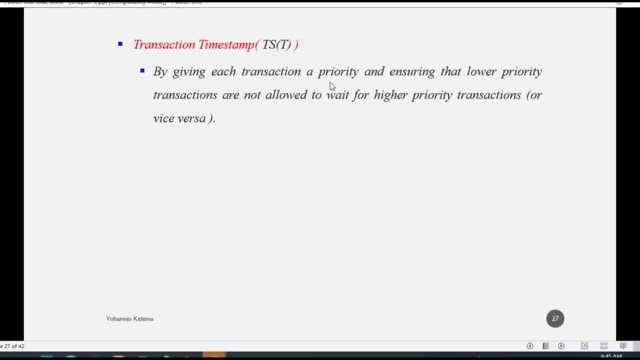 priority. set our malam by giving a transaction a priority and ensuring that low priority transactions are not a lot to wait for a high priority transaction where no vice versa man time sampling D email transaction which, in time stop, is a fat right. I am stamp the moment, Romeo guadalupe Marlena. I hope that you. 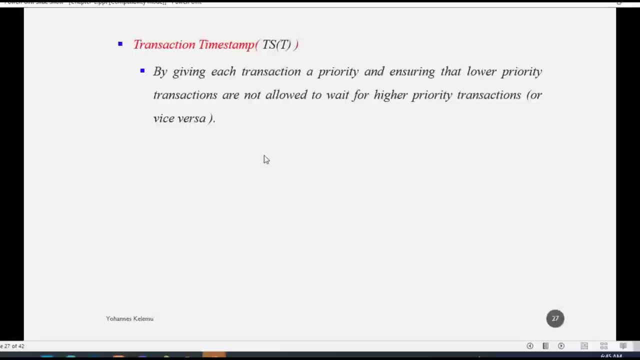 The priority is assigned to the transaction when the transaction is executed and when the transaction is not executed. One way to assign priority: it gives each transaction a timestamp when it starts up. When the transaction request is received, it is immediately sent to the system and the timestamp is assigned to it. 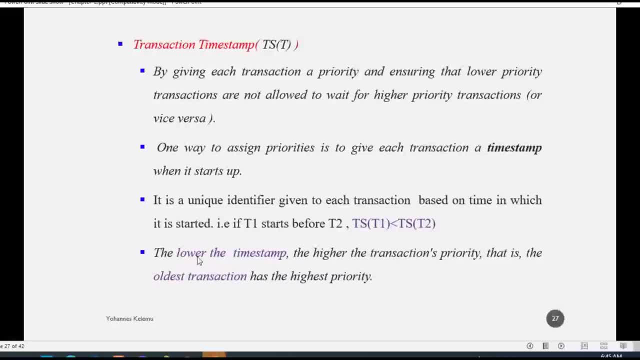 So this is a new technique called the low timestamp, the higher priority. This means that all transactions have a higher priority. The transaction timestamp has two and one techniques. When you apply the timestamp to a transaction, you will see that the transaction timestamp is the higher priority. 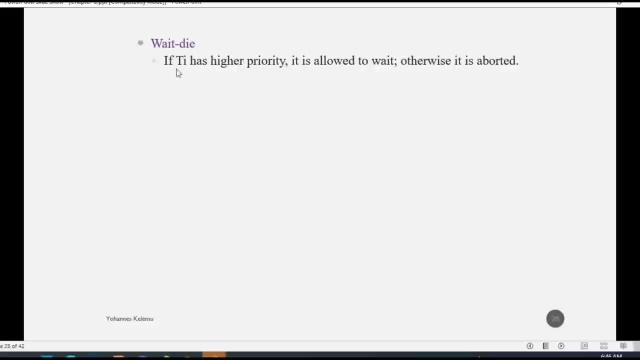 The difference is that if T1 has a lower priority, it will wait, otherwise it will abort it. When the transaction is high priority, it will wait for a while and then roll back. All transactions are allowed to wait for a while. When a transaction is low priority, it will wait for a while. 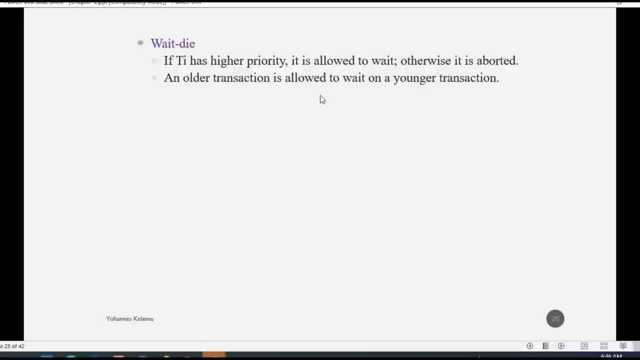 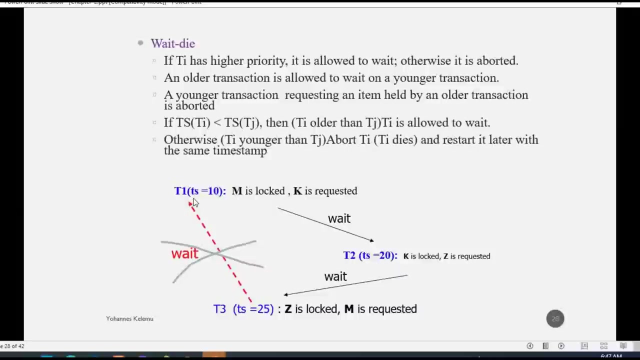 Young transaction request. an item held by an old transaction is aborted. The discounted transaction is known as the old item being held by an old transaction. The second is the weight die option. on the diagram, The time stamp of this product is 10 and the time stamp of the young product is 20. 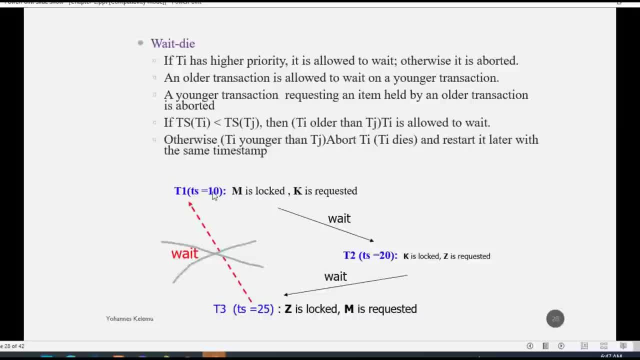 This means that the old item also holds the young transaction. The other one is another one and in case you are earning, you will be more likely to lose. So this is Young and this is Old, and Young will not give you weight. 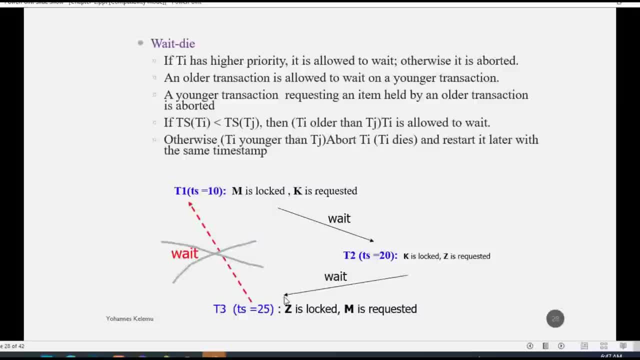 Here we have Transaction 2, and Transaction 3, where Transaction 2 is Old while Transaction 3 is Young, and Young will not give you weight. Transaction T1 is the old and the new one is the new one, so the new one is the responsibility of the old one. 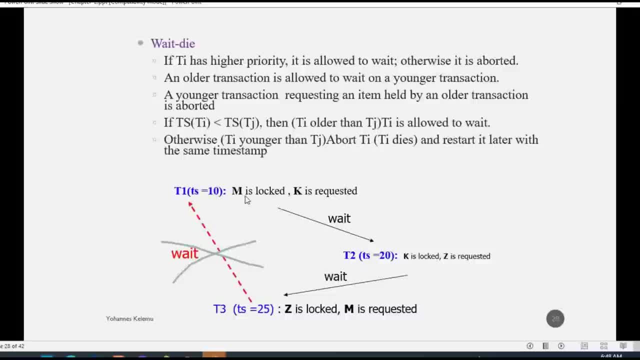 In this case, the Transaction T1 will execute the new one, The old one will execute the new one and the new one will execute the new one. The new one will execute the new one because the new one has high probability. In this case, the Transaction T1 will execute the new one because the new one has high probability. 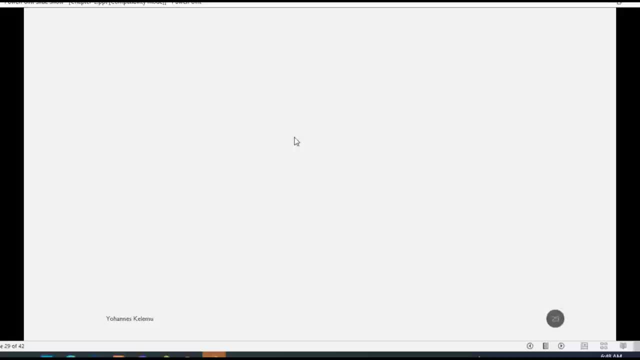 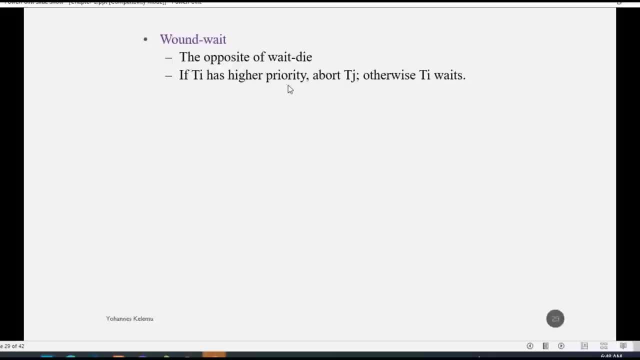 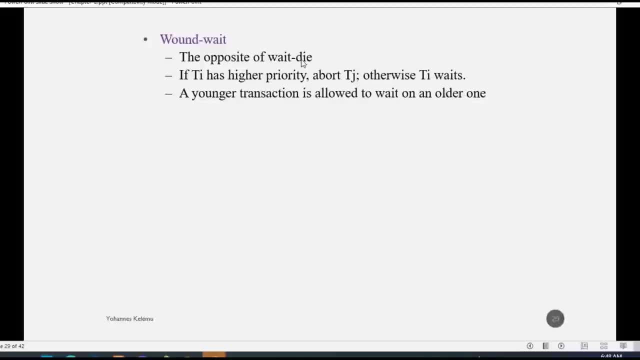 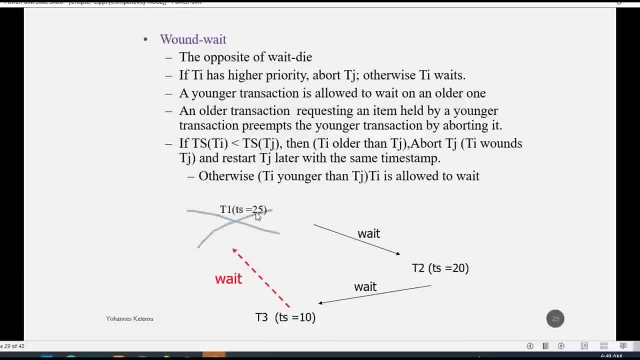 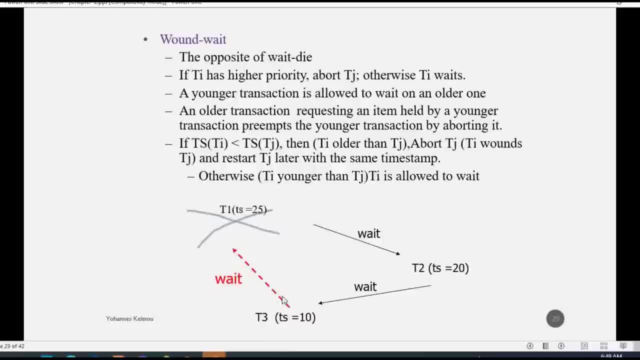 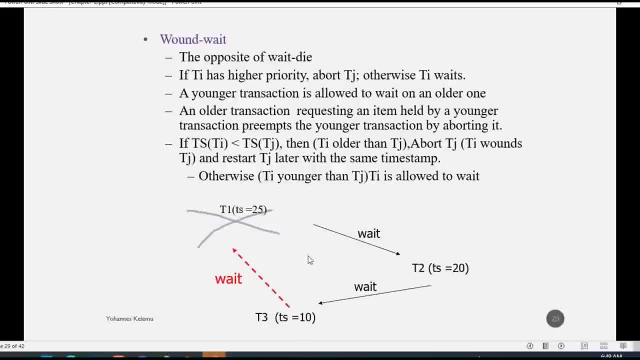 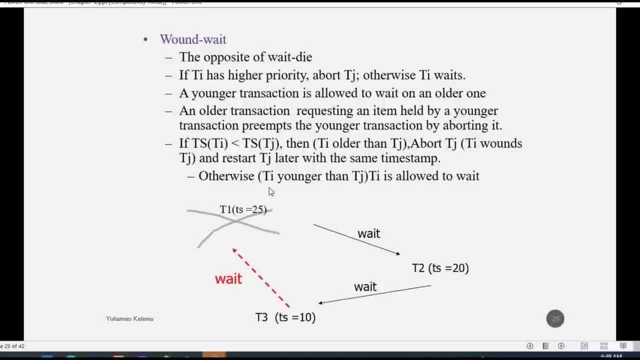 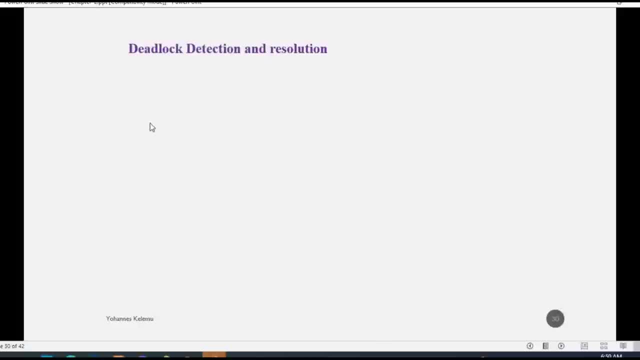 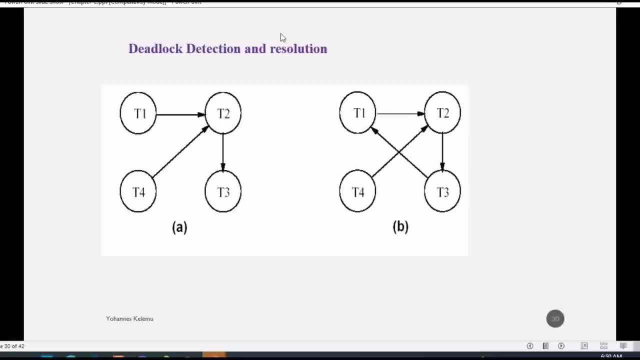 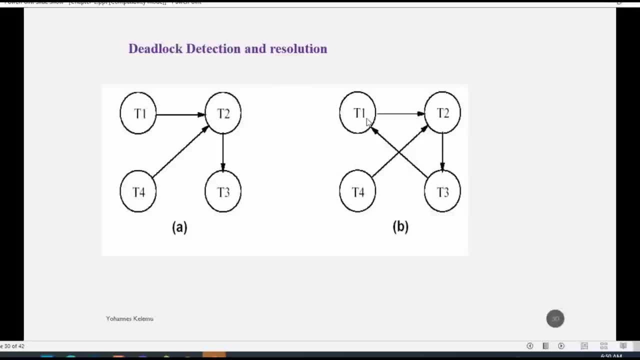 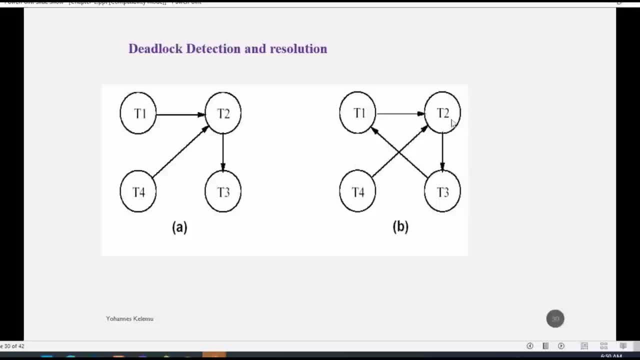 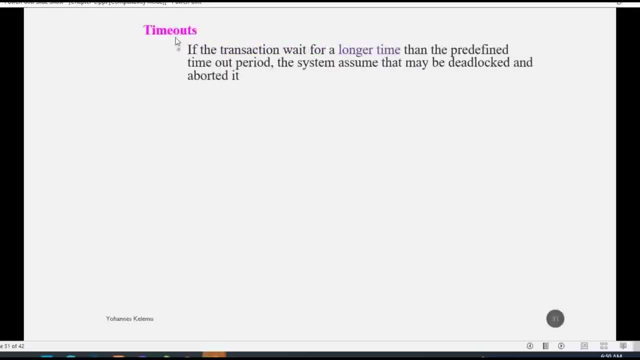 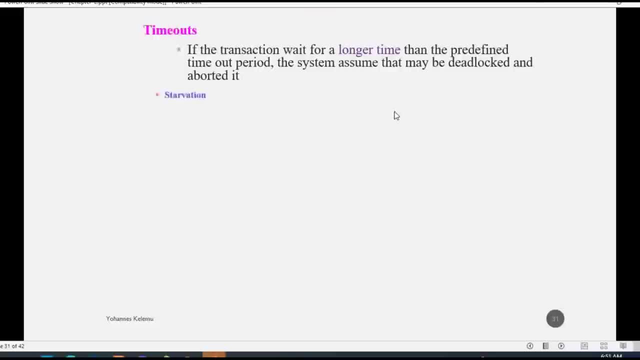 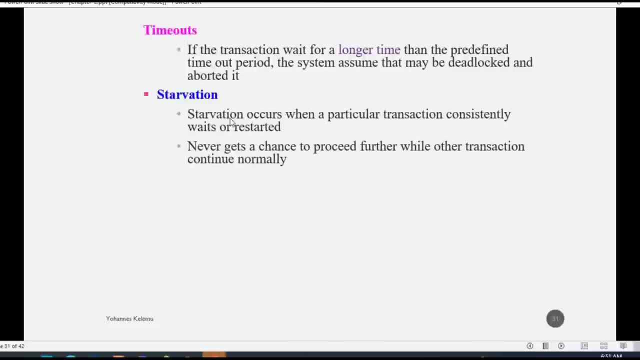 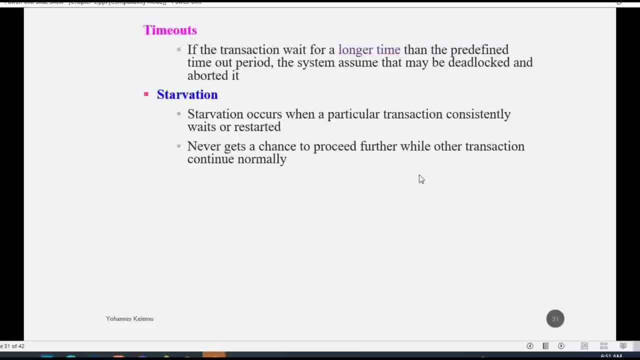 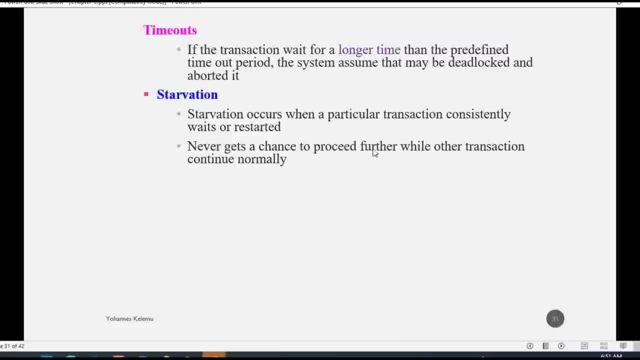 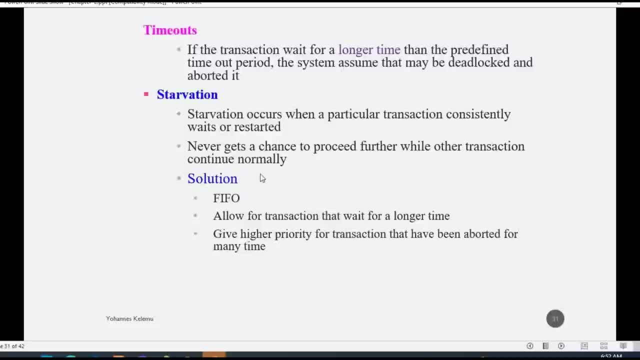 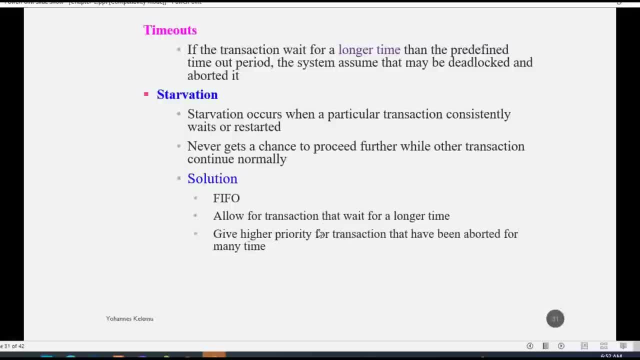 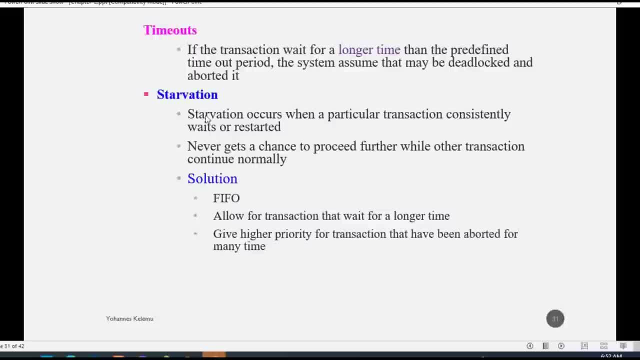 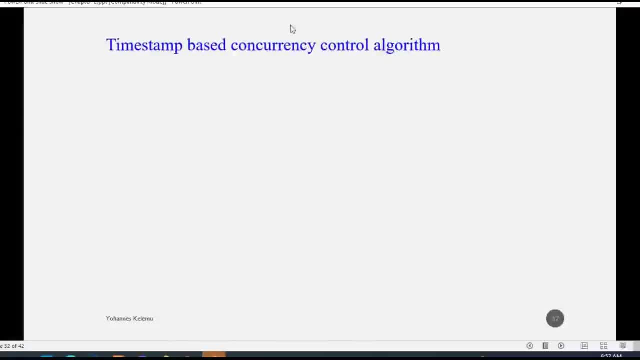 result: market in chile, malino. so Lela, no concurrency control algorithm on technique timestamp marathon only timestamp timestamp value assigned based on the time in which the transaction are submitted to the system using the current date. we have no more time of the system. gree a man, the new transaction. 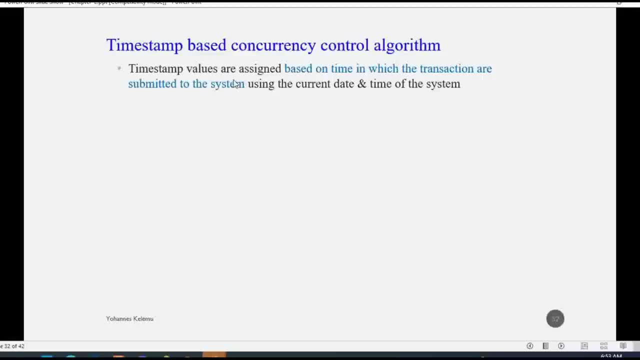 request for me. lack of exit. yeah, no transaction order system could get pop time. yeah, current day to win the way. a system on time, the medical timestamp set warm. I'm selling a request bleak and sell like a lock. we can decide the metal transaction, set the process at what will sound like a lacrosse, a tabloid. so 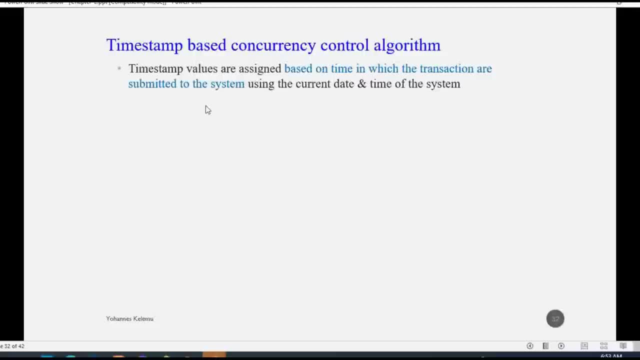 salita, alkyl, so silent. a blue metal razzle reset hormone, so lazy. yeah, time and no large timestamp. color value indicate the more recent even to a normal operation. Marlon, I'm sorry. timestamp one and a timestamp to install timestamp one. can we met our timestamp to can own recently met on a blue system we. 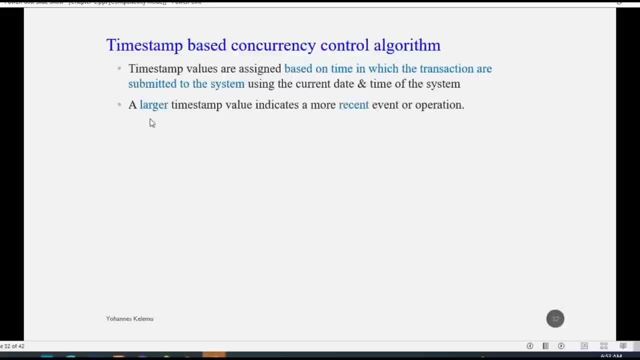 mirrored a sleazy timestamp, one much of an execute, a regard as a timestamp to cut to the other galvanized lady and a meta-touch or the transaction which minister timestamp messed at my last night. timestamp based algorithm use timestamp to serialize the execution of concurrent transaction. gree, a metal. 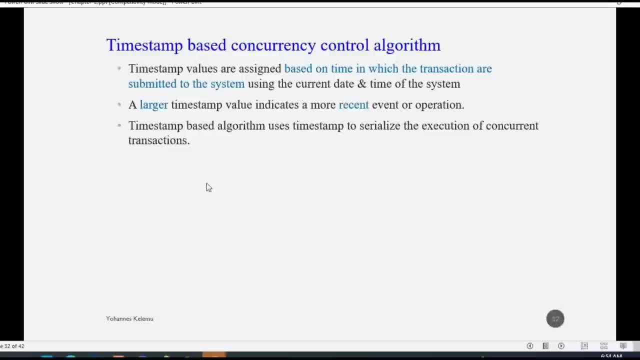 transaction serialized. Lee, excuse me, derogu, yammer, gnomar and a meta-touch, oh time is a touch. one selling the transaction one, but in service, or transition to by the status or our murder. so can mo execute our God? you mean concept and you know ratio, Malino's lazy in timestamp that does not have the look women look. 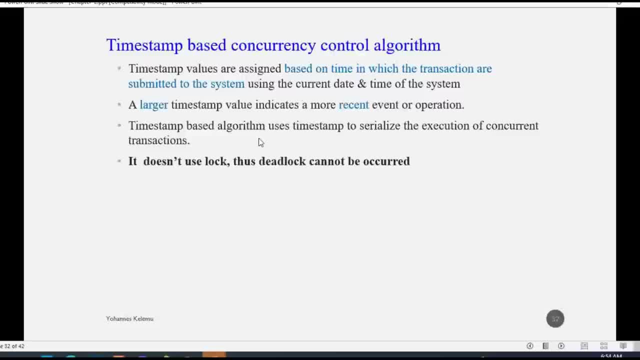 saline. deadlock me, found problem. I got on Kato not a touch. oh, time set. oh, I tell me I'm just going darago Marlon on J lock and lock me. panickingczenie leded. look me, found problem. in the timestamp lie a modern. No, so I'm gonna. 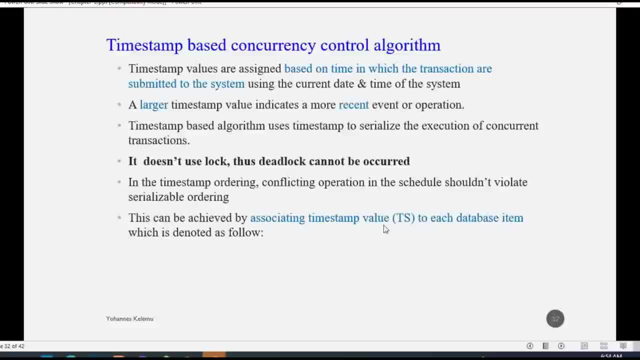 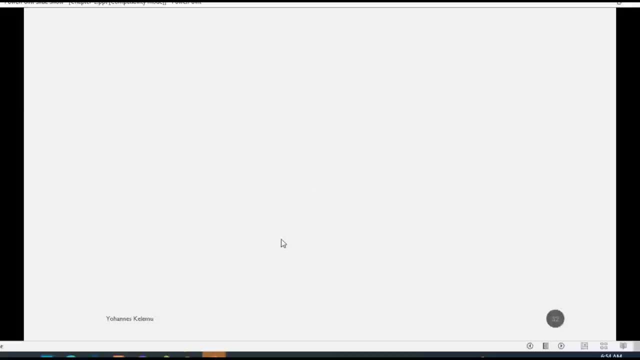 So they can be achieved by associating timestamp value to each database item, which are denoted as following: The first item is executed by the timestamp value read the timestamp of x, that's the largest time among all the timestamps of the transaction that have successfully read item. 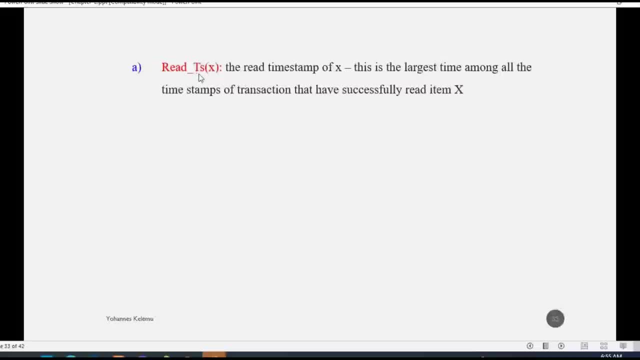 x in the same format. Also, the priority of read item x is that transaction x is executed in the correct way. Why? Because transaction x has a large timestamp. The right side is the same. If x is not read by t, then t is large timestamp. 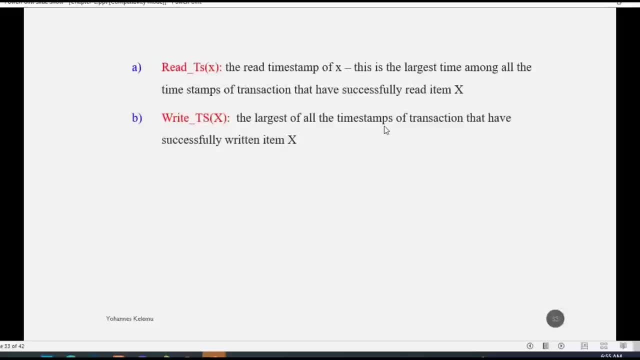 That's right If t is large timestamp. Now let's look at the time stamp. The important thing about a transaction is that it has to be executed. In a transaction, high priority means that the transaction has to be executed. The high priority means that the transaction has to be executed. 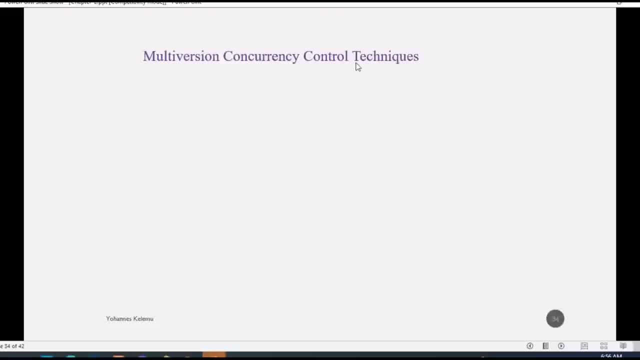 This is a multi-version concurrency control technique. The number of versions of that item is allocated, the right version to read the operation of the transaction. Now let's look at the Bürger Mask, For example. this is a Vol remains X item. 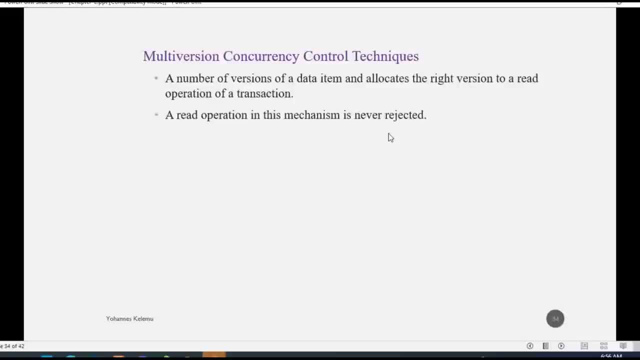 Then it is called multiple copy item. This is X item and then a copy X1 touais to X3 copy is extra copy. For example, this copy is outside the lane where the transaction has to be executed In commercials. Shaun Bad Kim comes to the избéraloo. 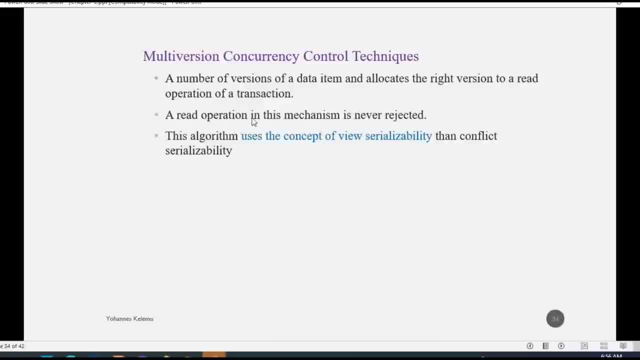 outlook. none Slice in design operation, line read operation in this, the mechanism to never reject a direct marital and one no X, look bitter ragam when one no X or a developer transaction be asm yes, yeah X and copy members limit. you know a read: never reject a direct man, never reject a direct, like this algorithm, you the. 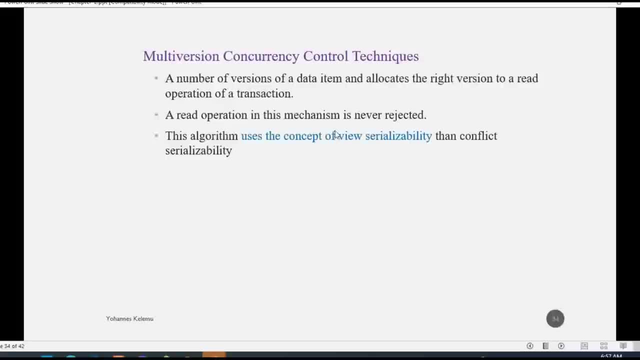 concept of visual serialization. no, me, take a move, view serialization. take a moment on conflict serenity. you know conflict to like transaction part to video item. you serialize even multiple, no complex analysis, multiple, milo, slazzy, multiverse, like the view as realization. most important of that: um copy, slow, normal director copies for a. 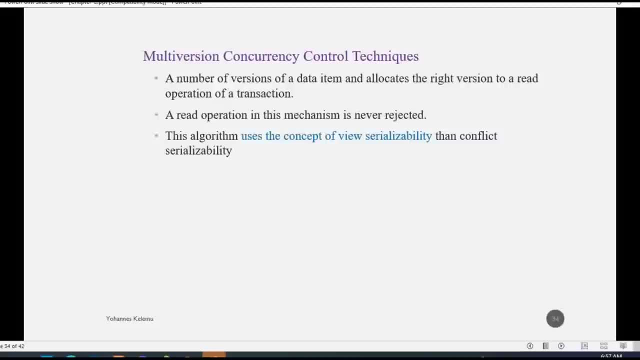 view X do like my attention and the modern. no okay, green side effect to the nose. you got multiverse, July and more storage. if any kind of atom X equal data, call a as an X data in a multiple copy. produce by my record back, see Ram webdisk. if any kind of art, no slazzy, I'm under, no more. 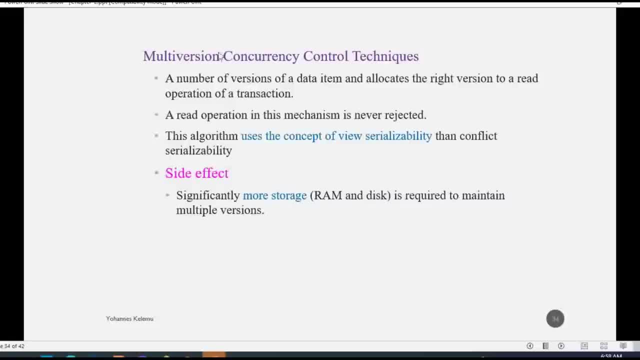 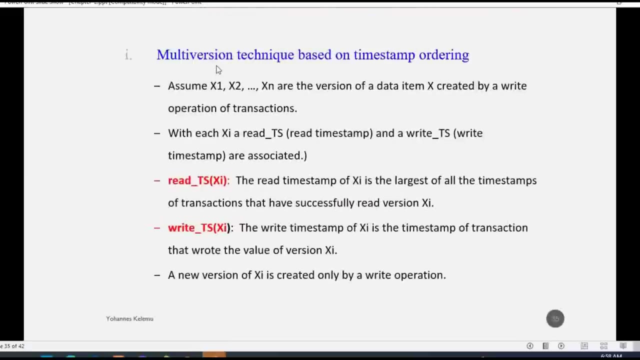 storage waste, another got them out. no side effect to a multiverse inside. fake, you know, slazzy the multiverse in. apply the maric time stamp. a match, a child, a more to face local met a commercial aluminum, as you guys. examples in alignment version: timestamp an example. 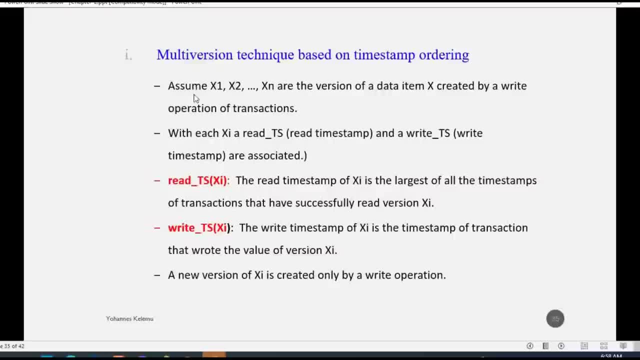 and elements. I assume X me Polite am. I mean let's a X in private, an X 1, X, 2, X n me Baldwine has committed, let that low invalids has committed right operation and then I take a ride or push in the meta, come he is, a version has committed. 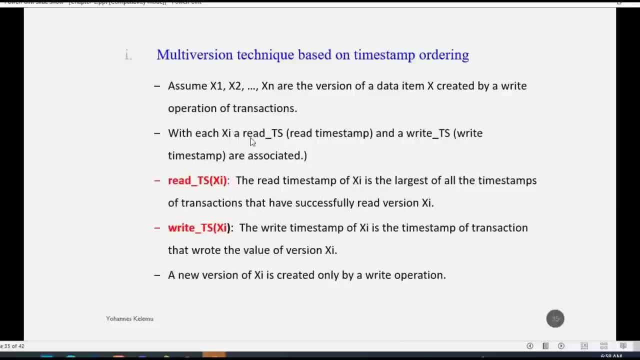 let alone. well enough, now sazi with H x 1301. the transaction T s min man X n reads magic. a fan leggerụcr X could have the birth. little too nice in version. read never reject. read transaction s x1 and x2 read. 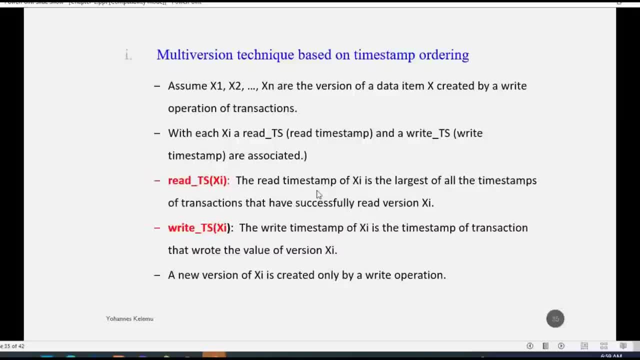 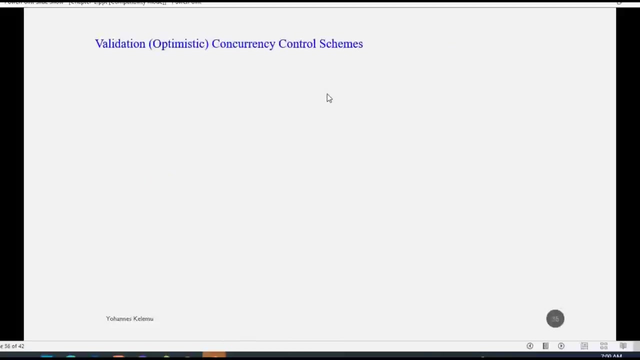 timestamp x1, x2, x3, x4, x5, x6, x7, x8, x9, x10, x12, x13, x14, x15, x16, x17, x19, x20, x21, x23, x24, x25, x26, x27, x30. 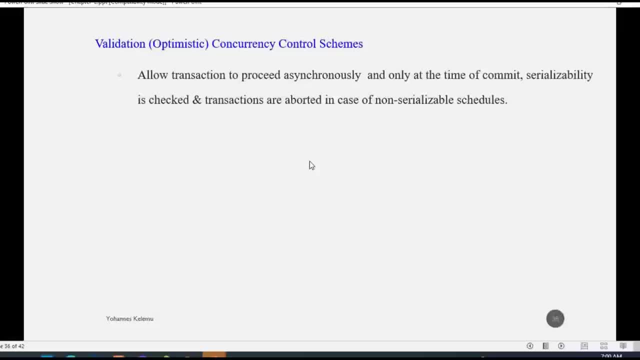 x31, x32, x33, x34, x35, x36, x38, x39, x40, x41, x42, x43, x44, x45, x47, x48, x49, x51, x52, x53, x54, x56, x57, x58, x59, x60. 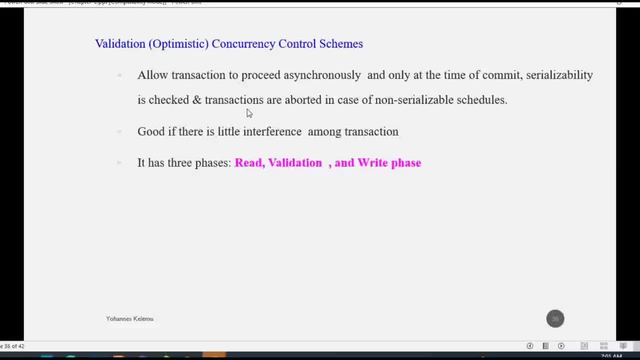 x61, x62, x33, x33, x34, x35, x36, x36, x37, x38, x39, x40, x42, x43, x44, x44, x45, x46, x47, x48, x49, x50, x51, x52, x52, x53. 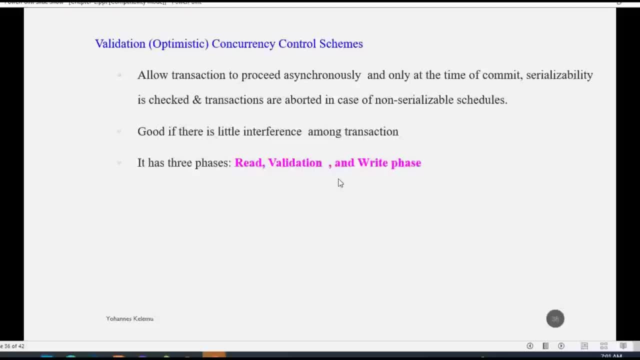 x54, x55, x56, x56, x57, x57, x58, x58, x59, x60, x61, x62, x63, x64, x64, x65, x67, x68, x68, x69, x70, x71, x72, x72, x73, x73. 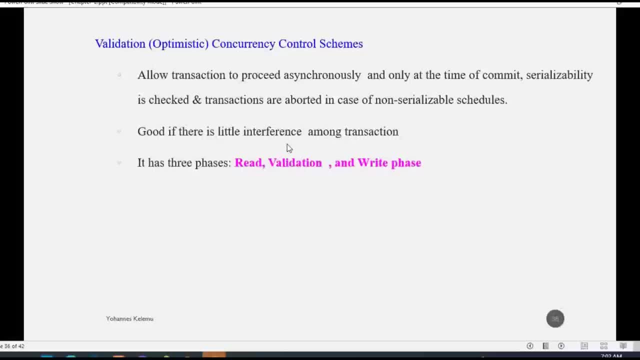 x74, x74, x75, x76, x78, x78, x89, x90, x90, x92, x93, x94, x95, x97, x98, x95, x99. seeing 00, 4, 13, anything back, x97, 18, 18, 20. 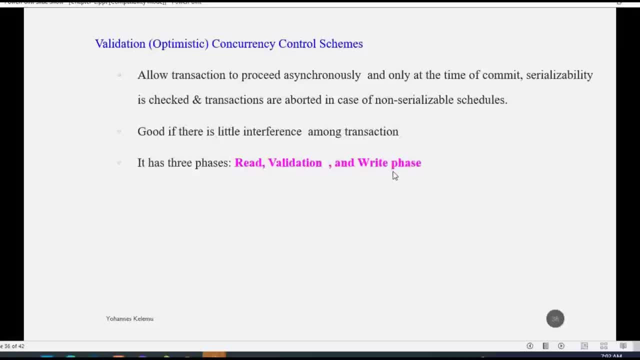 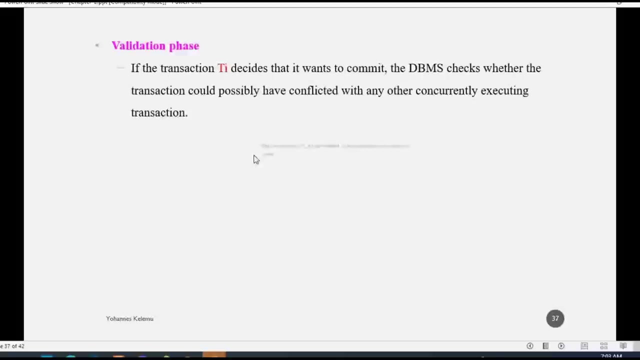 23, 23, 24, 26, 24, 24, 26, 27, 28, 27, 28, 29, 30, 30, 21. This is called optimistic Validate here with the transaction at the transaction table. We can check the transaction on the right side of the screen. 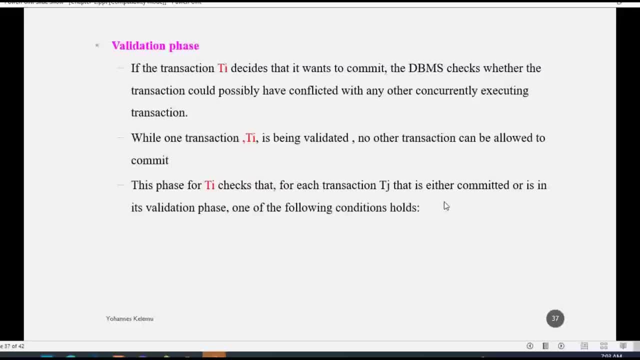 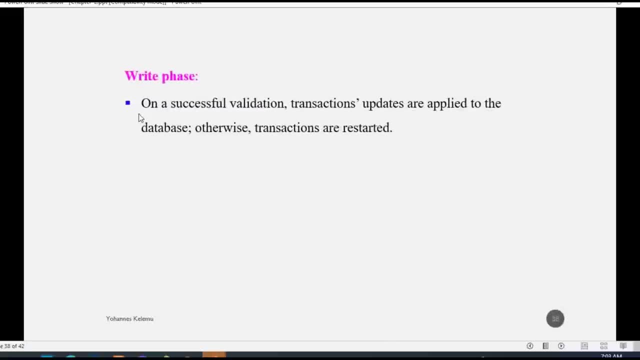 After checking the transaction, we can go to the right side of the screen. After validation, the transaction will be updated directly to the right side of the screen. After validation, the transaction will be returned to the right side of the screen. We can see that Optimistic is using the same technique. 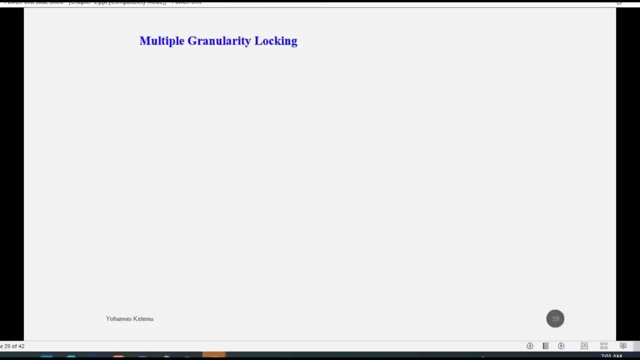 We can see that it is using multiple granularity. We can see that it is using multiple granularity. Every unit, for example A and B, is used to log the transaction data. We can see that it is using multiple granularity. We can see that it is using multiple granularity. 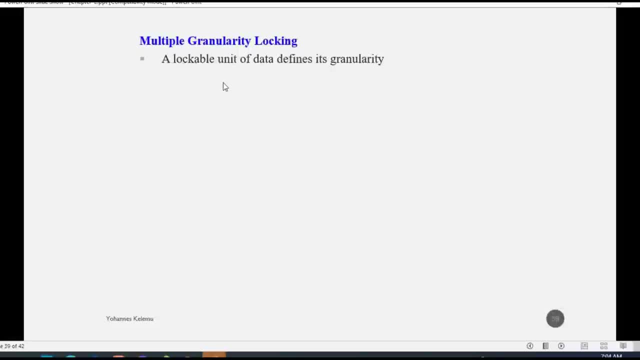 As you said, we can easily identify any part of the unit of data. the concept of multiple data looks. another minute point: the metal in a mirror, it can be this side in that database. look when, the more it can be fine attribute: look, we know more relation, look. and then minute concept: no, me metal. 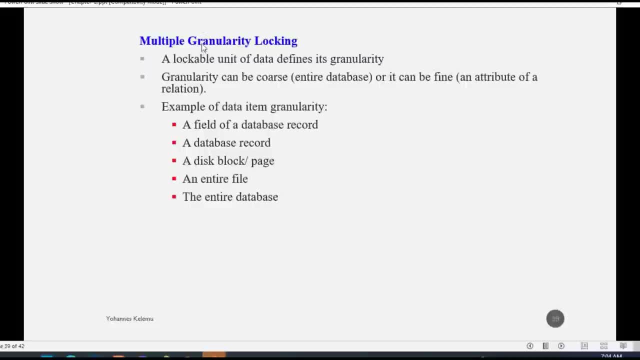 in the middle in me, as I, you know so multiple grand art, local angry. that item, grand alchemy, know that field, you initial database, you initial database. when we cut you in child, this conventional entire file which shall enter that have is going child nazi man named Paul, ground ready to know in Paul. 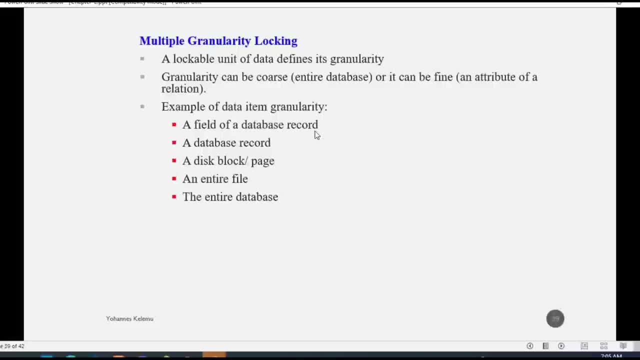 Donald is lazy and transaction doesn't have a zoom. data is a record room. look like a child fit in. look like a child- this couldn't look like a child- entire file. look like a child, entire data we zoom. look like a child lazy, does it matter? go ground rarity technique in. 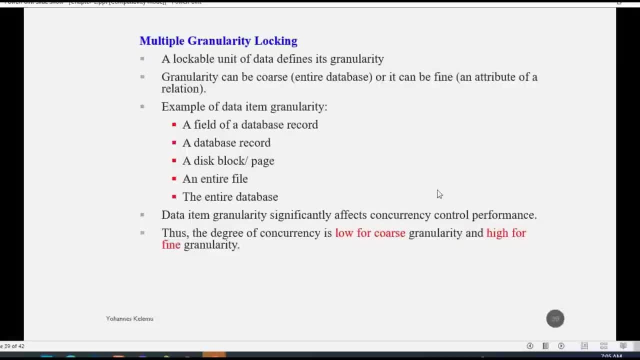 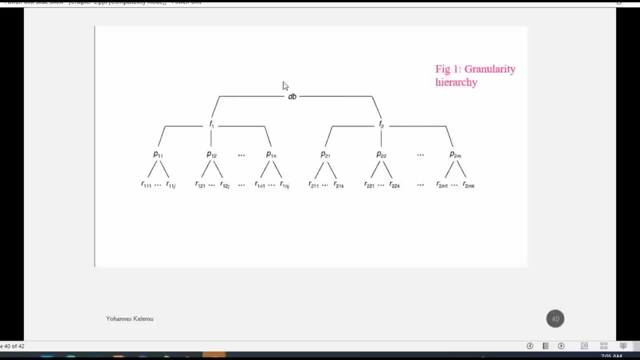 tatak mo look muddick much on a child model. no, so I'm gonna do my name. sorry, Zika, but yeah, grab last. I got you a database. no database on gree. it like phil, go charlotte field, one field, two field, three. a little child, feel good. 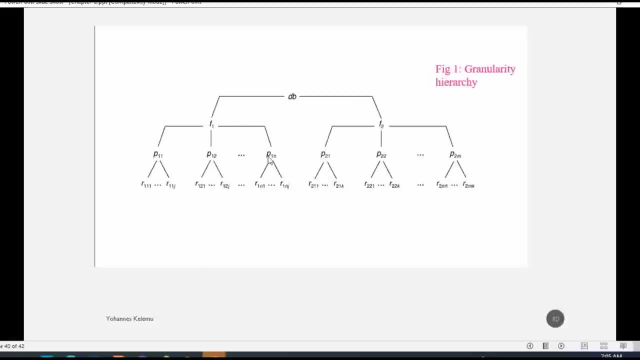 you know material record wrote you know what I'm files my life. I wrote you know what I'm nazi files to material record wrote you know what's true. record was a transaction method outside reason is Dolores much more than we know and transaction method siloed. 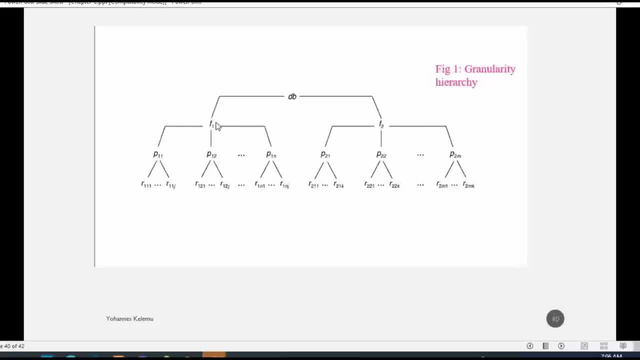 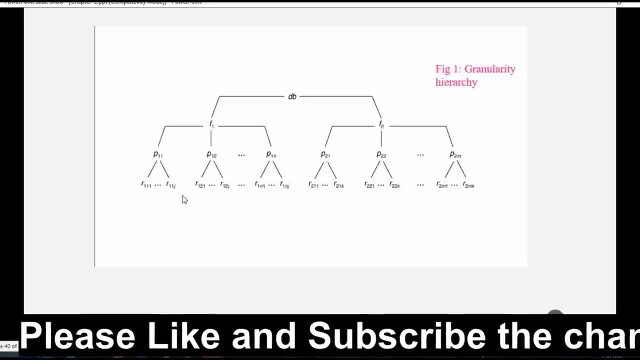 look mother in child file and Moodle locator, girl Zega, working of which in Meta game: child women transaction. better record Moodle: yeah, I mean filter chin. look material وجillan locator: yeah, Wallah moon, as in a record wrote: excuse, mother, yellow mother turned out to be the other one that was written in record to. 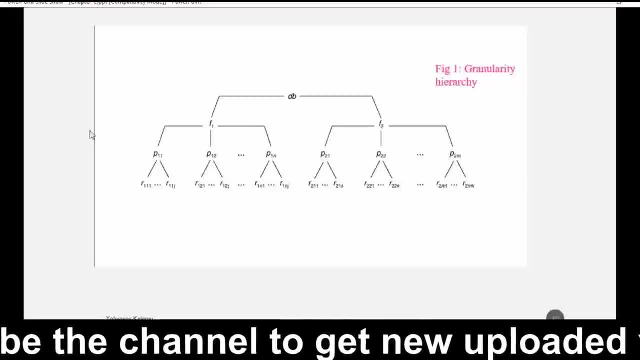 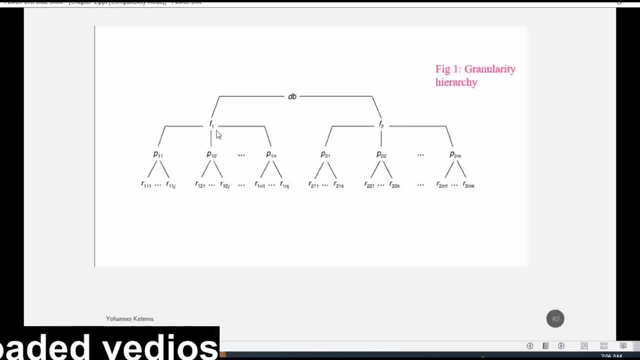 So we have two levels. First, we have the file that we want to use. Second, we have the file that we want to use. Third, we have the file that we want to use. Fourth, we have the file that we want to use. 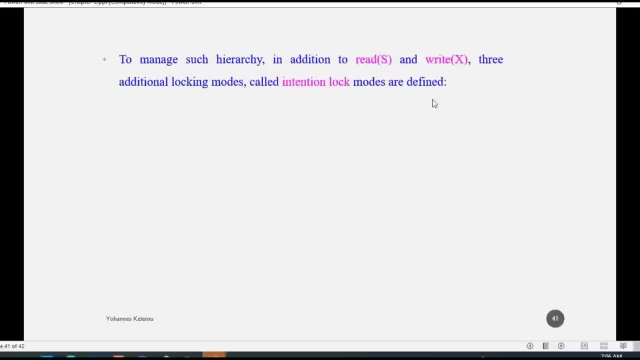 This is called Ground Reality Lock. So what is Ground Reality Lock? It is an Intention Lock. It is a specific item lock. It is a read lock, write lock, exclusive lock and shared lock. It is a read lock, write lock, exclusive lock and shared lock. 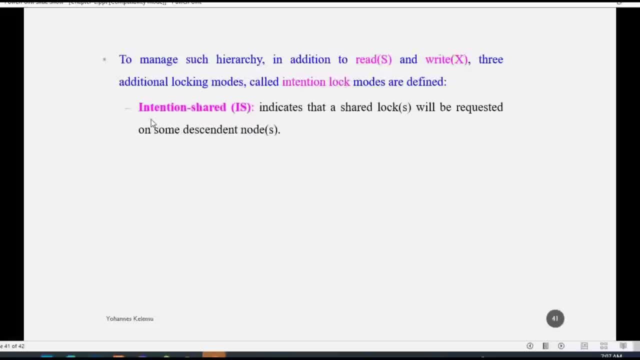 So in Ground Reality it is an Intention Lock. Intention is a shared lock. It is a file with a decent node. Shared Intention is an exclusive lock that applies only to the descent node. Shared Intention is an exclusive lock. 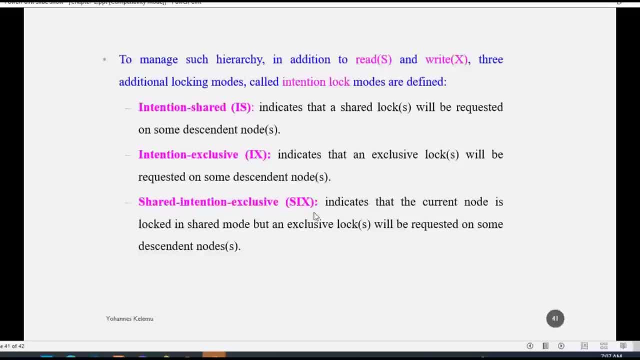 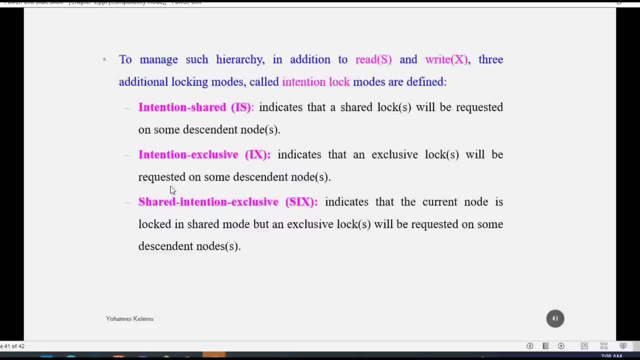 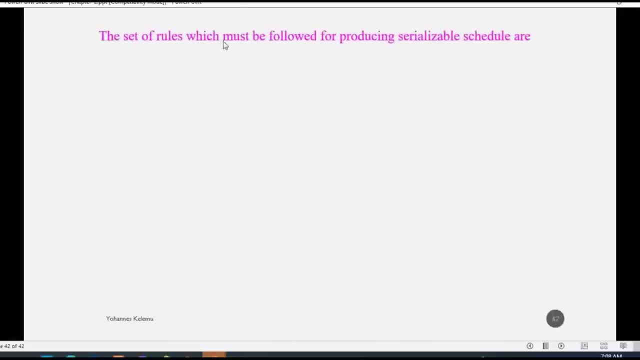 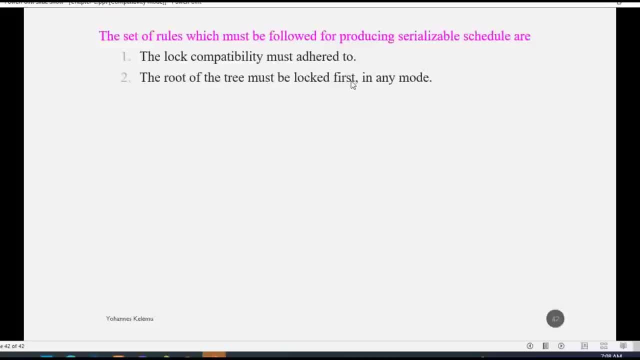 The root log of the tree must be logged first. For example, if you want to access the file, you have to log the file. Then you can access the record. The second one is to check the log compatibility of the tree. The root log of the tree must be logged first. 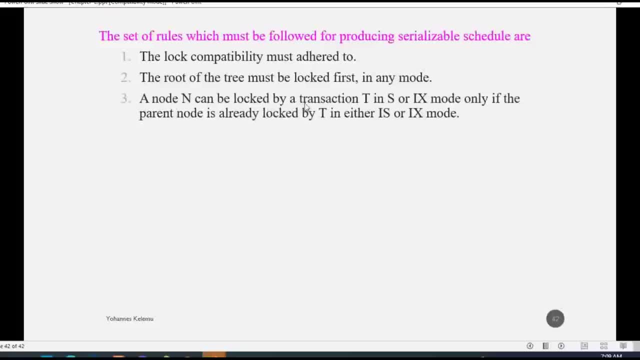 For example, n nodes can be logged by a transaction. The root log of the tree must be logged first. The parent node must be logged first. The exclusive log must be logged first. The exclusive log must be logged first. The parent node must be logged first. Then click on the n node to change the access. 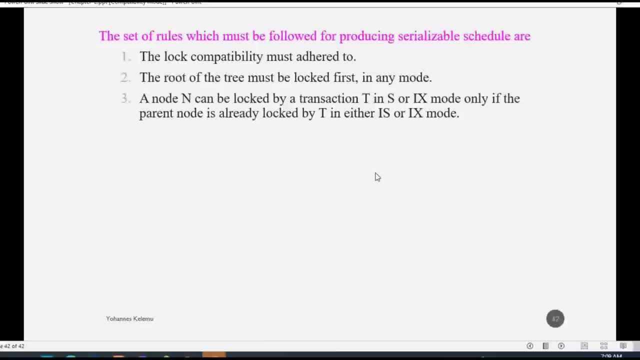 The parent node must be logged first, Then click on the excute. The n node must be logged by n monopolies. So if you want to use a lock, you have to use an exclusive lock or a shared exclusive lock. So if you want to use a parent lock, you have to use an exclusive lock or a shared exclusive lock. 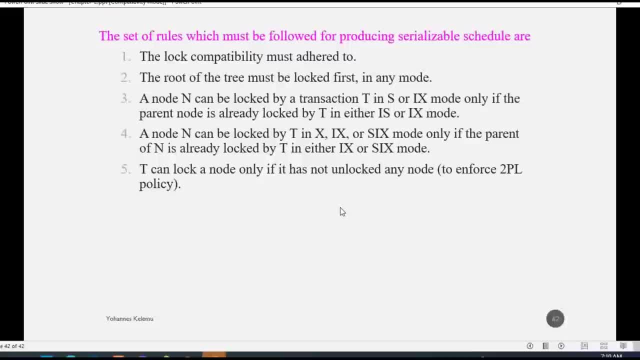 You can't use that lock, so you have to use a ruler. You can apply that rule. so that is an example of a parent lock. that means that its an exclusive lock. Now let's add an exclusive lock. We added a parent lock. 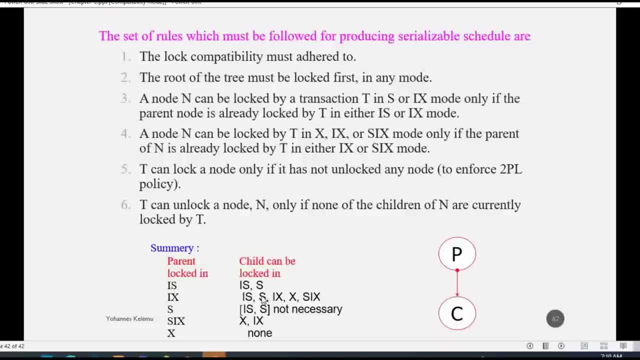 So can you see the rule: child look located a gamma Z gamma to a show: exclusive look, Carly, I'm Sally, apparently exclusive look at the gala because a child like exclusive look when the motion look at the gala- no, as Gala, I mean shut- look at the guy could. 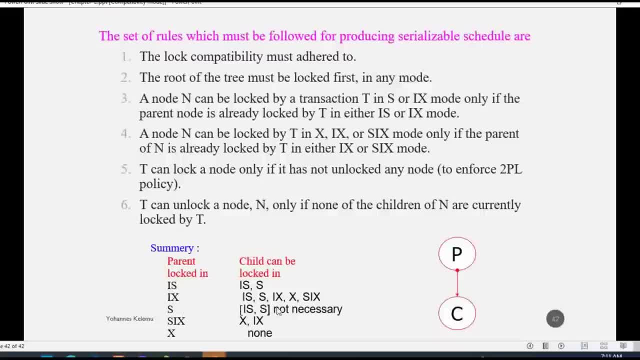 exclusive look at a exclusive look, greater than the shirt. look at the gala: the child like nothing got you. look at your play market. each another model. no, let's see. let's see what's not so like grand ralph's local limit taken when I need to apply my record below, yes, I, you know. so let's see who lay child look and. 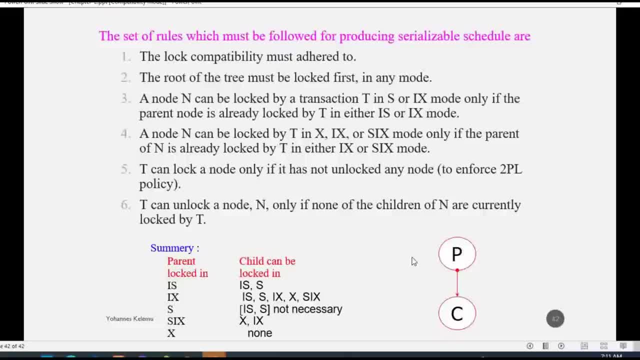 look Lamar the child, look at an access. Lamar, a parent. look my mother got a bit. look my daughter got a body, a granite, a rule: yeah, man and I'm data. look America, but see, apply a man. undergo main rule: parent: look first. look at a garden, try it in.